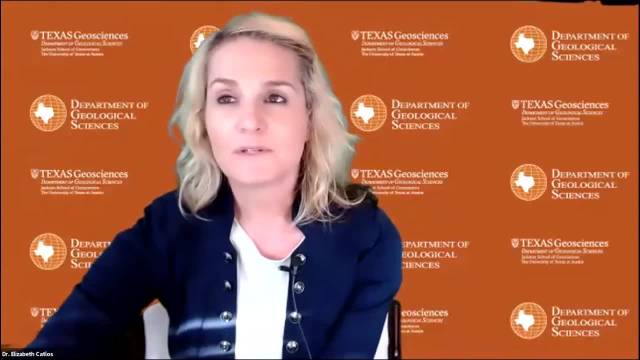 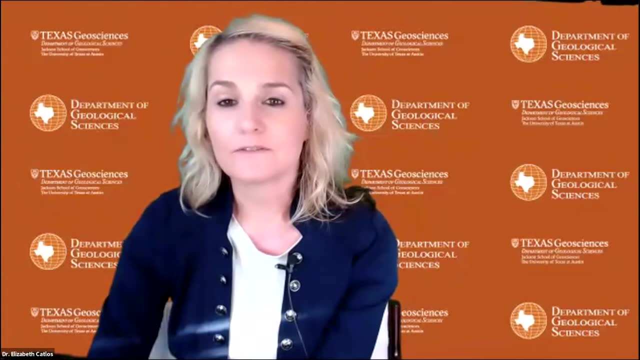 Lecture Series is our departmental seminar series. It's been a requirement and tradition for all graduate students since the late 1940s. The lecture series is named after Professor Ronald DeFord, who joined the University as a professor in 1948 with the purpose of enhancing the quality. 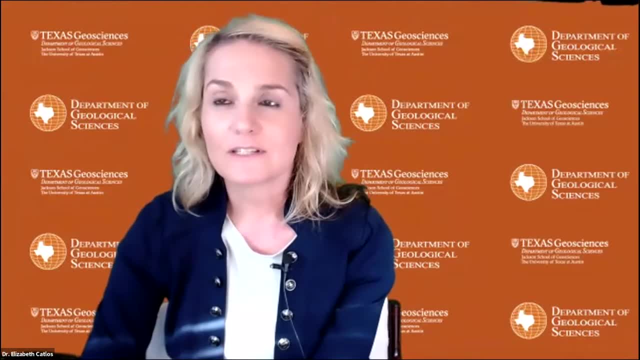 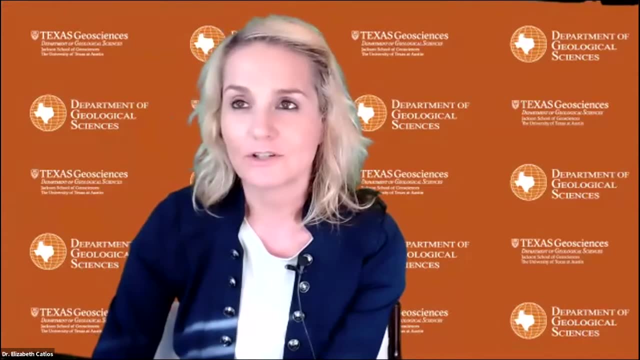 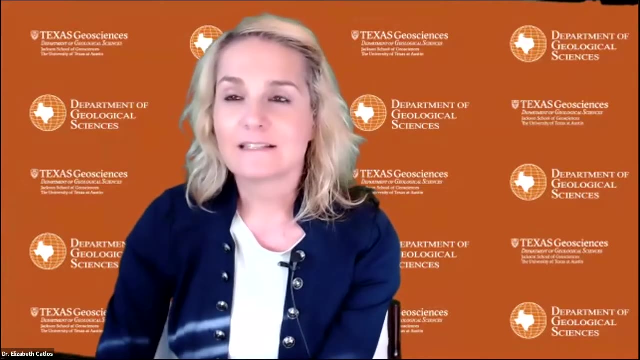 of the graduate program of the department. Our lecture series is supported by a series of endowments and today's speaker is the Fred L and Frances J Oliver Lecturer in Texas Hydrology and Water Resources. The lectureship was created in 1985 and this speaker will be our 35th, Oliver. 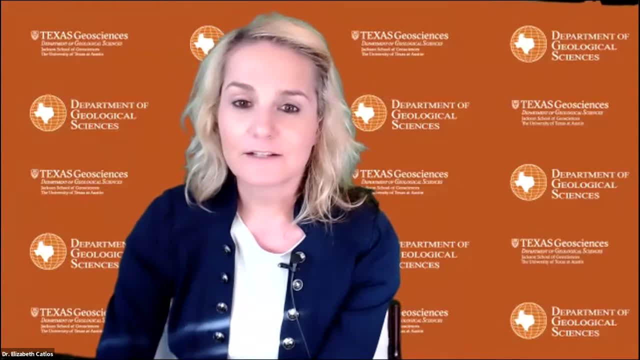 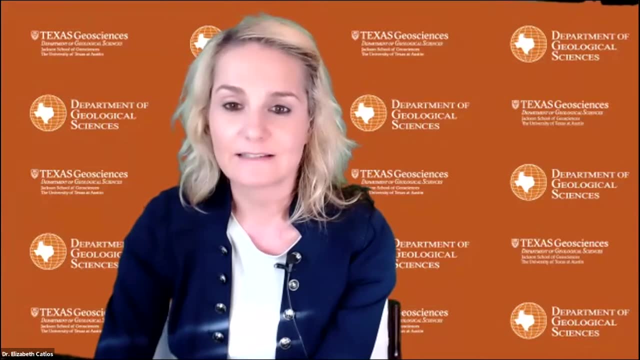 Lecturer Fred and Frances Oliver created the lectureship because they were so passionate about the topic of water, and they were so passionate about because they believe the study of water resources in Texas is as important as the development and exploration of oil and gas. They established the lectureship with the goal of providing better 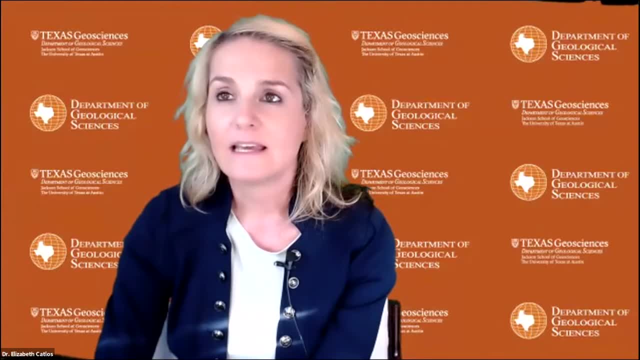 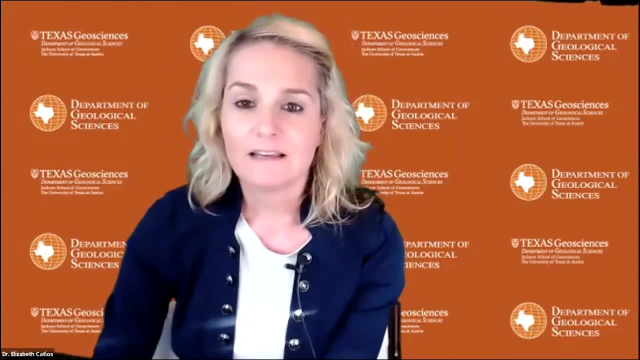 education concerning water problems being faced by Texas and solutions to those problems. Fred received his Bachelor of Science in Geology from the University of Texas in 1951. He's a current member of the Geology Foundation Advisory Council. He resides in Dallas, Texas, where he's president. 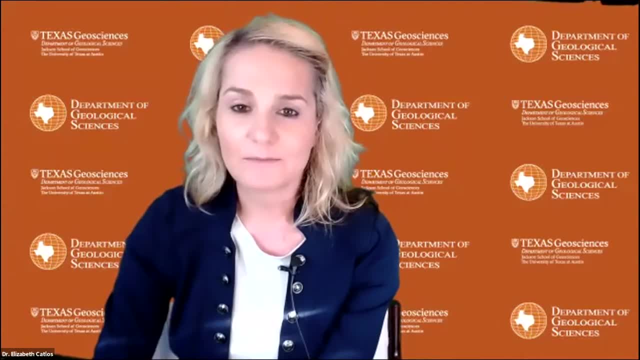 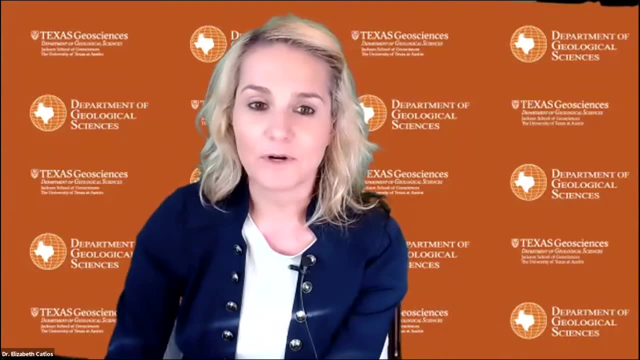 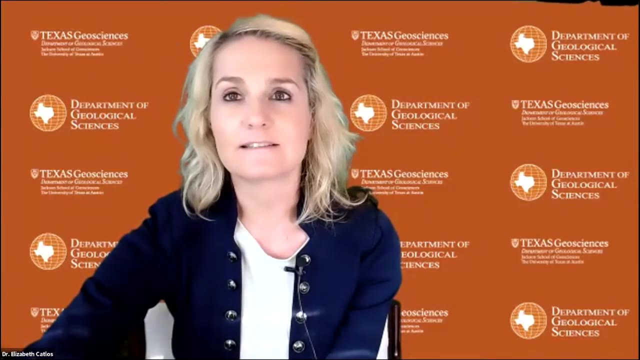 of PVT Inc. In 2009,. Fred's family established the Fred and Frances Oliver Endowed Scholarship in their honor to recruit graduate students into the field of hydrology. Our speaker will be introduced formally by Dr Dan Breaker, who's an associate professor in the Jackson School of Geosciences. Dan 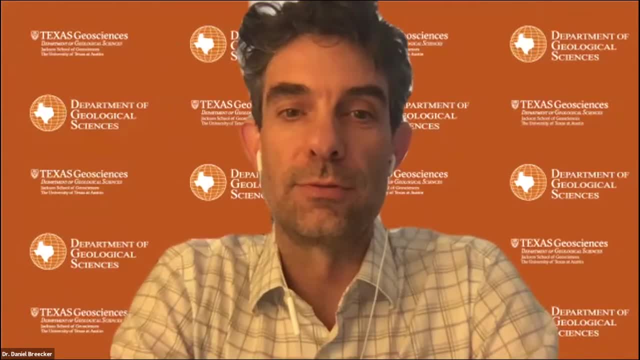 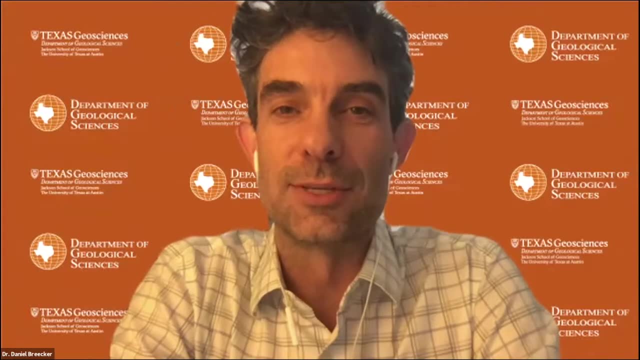 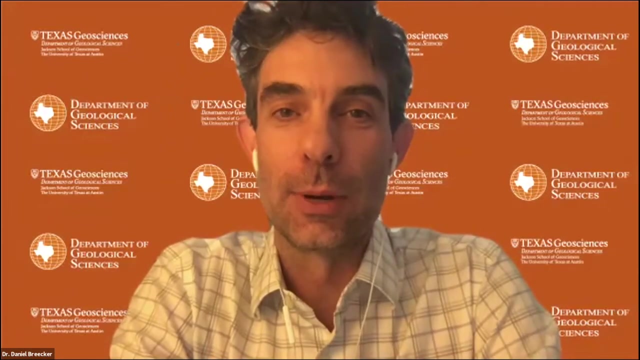 Thanks, Liz. Jerome comes to us virtually today from the Institut de Physique du Globe de Paris and it's late in Paris, so we need to thank him especially deeply for joining us. Well, Jerome has done quite a lot with his career, but some of the highlights here: 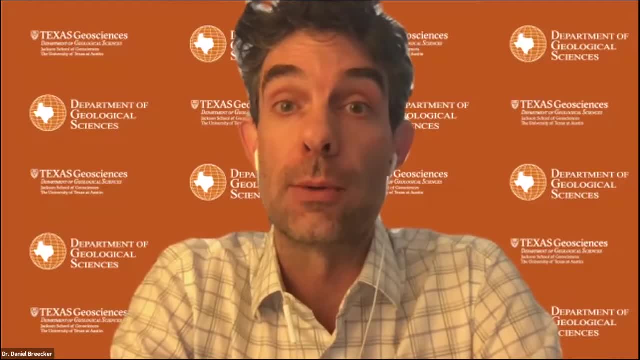 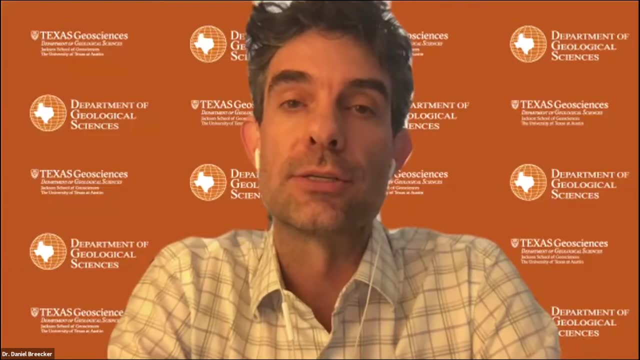 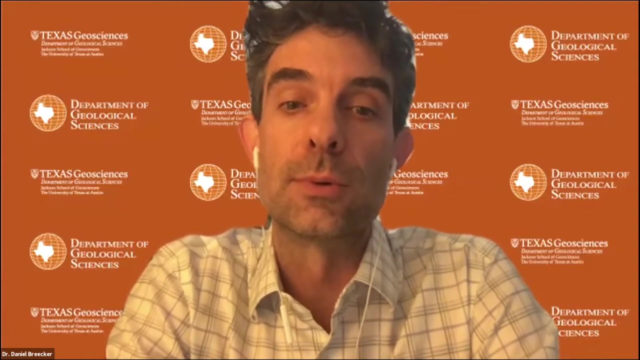 are that he has coordinated the French network of critical zone observatories, and he was also awarded a medal from the French National Centre for Research, the CNRS, for the quality, originality and the importance of his work, and he's also a fellow of. 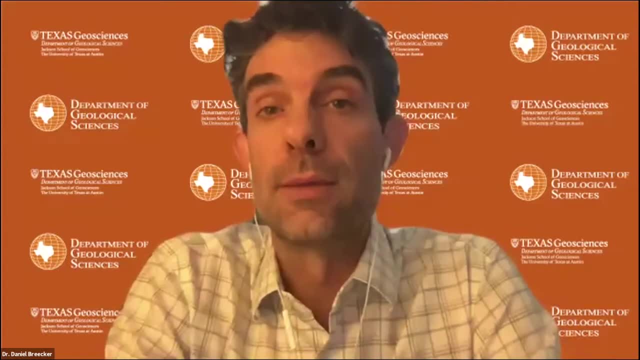 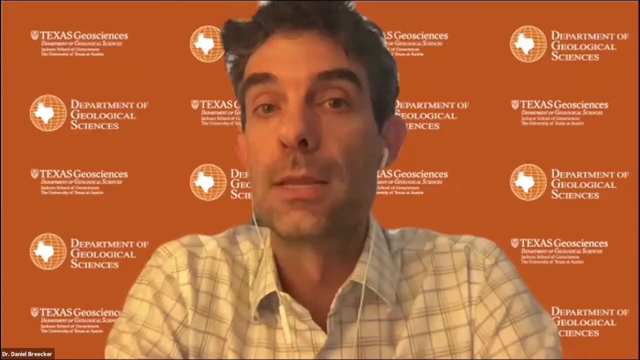 the European Association of Geochemistry and of the American white Louise tailleur study and of the American Geochemical Society, And he's going to talk to us today about what he's perhaps best known for- the geochemistry of rivers, And Jerome is really a world leader in this field. 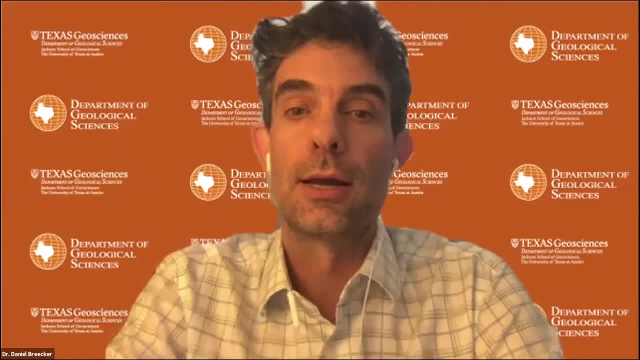 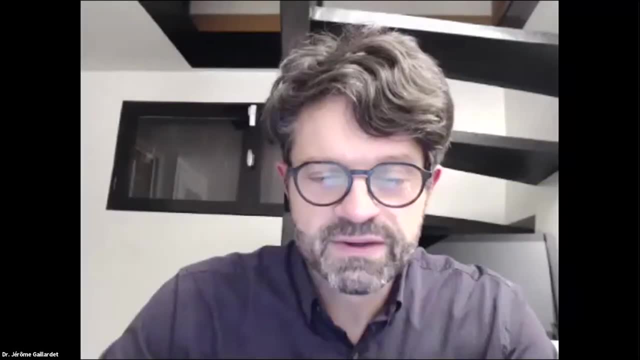 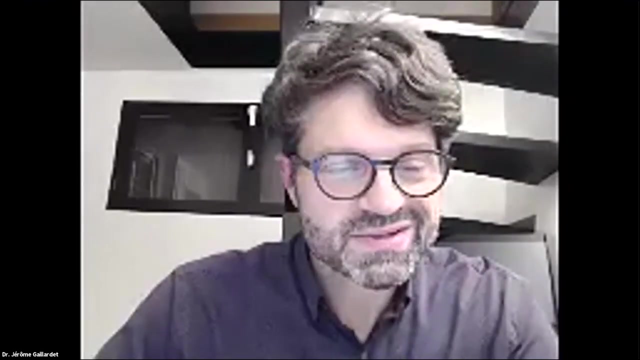 and so I think that we're all going to enjoy his presentation very much. So thanks, Jerome, and I'll hand it over to you. Thank you, Dan. So thank you for the invitation. I must say I was a little bit surprised of the time of the presentation. It's the first. 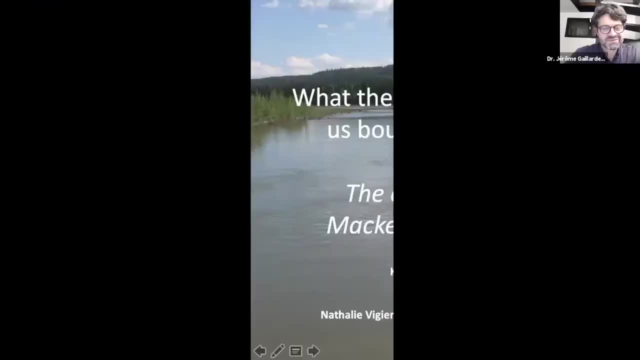 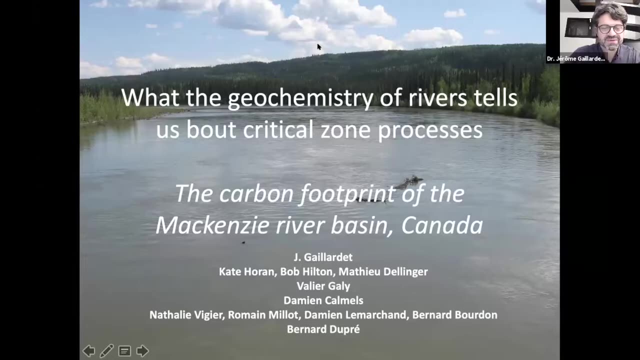 time in my life I'm giving a talk so late, so please excuse me if I say strange things, It's due to the hour here. So initially I gave a title to Dan which was about three: what the chemistry of rivers tell us about critical zone processes. And while preparing the 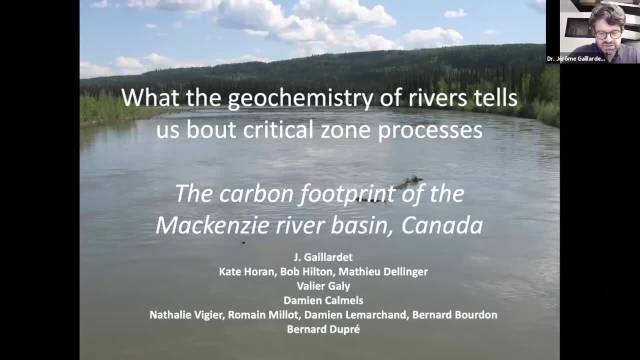 talk, I realized that I was probably too ambitious, so I have restricted my topic today And I will talk mainly on one application actually of river chemistry, And I will take the example of a recent paper that we have been published, which is to establish the complete mass carbon budget of a big watershed. 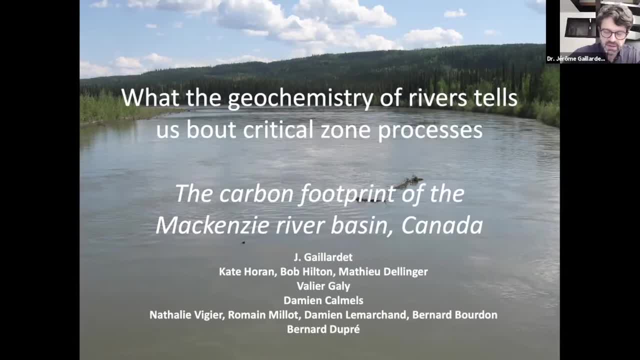 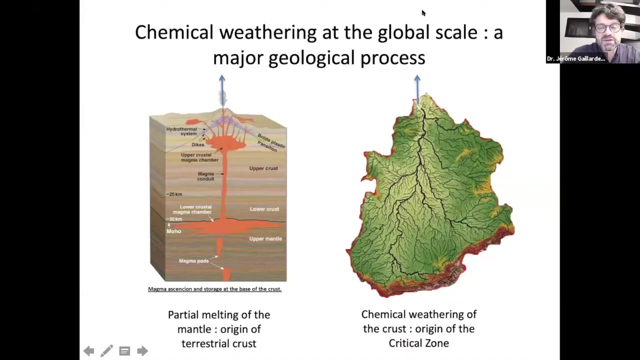 which is the Mackenzie River Basin in Northern America. So I'm still talking about the geochemistry of river tonight, but I will restrict my topic to the Mackenzie River Basin. Okay, So Dan, tell us about the tubular layer. So 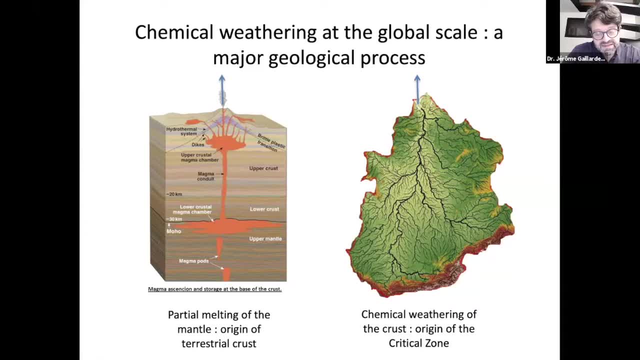 it's called the Basin River Basin. Basin Basin rocks have been studied by geochemistry for multi decades to get information about the mantle and the partial melting of the mantle and the, the, the. the philosophy with with which I've been working so far is to use rivers in the 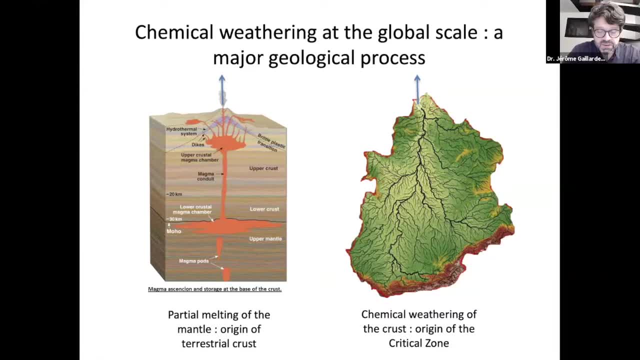 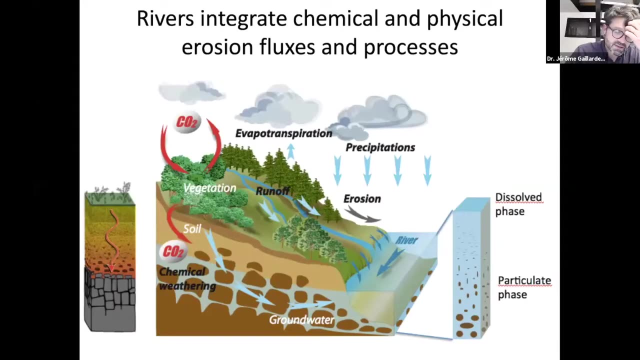 same way to gain information about chemical weathering of the crust and basically to understand the the origin of the critical zone. so I have pronounced the name of this thin layer at the surface of the earth that we call the critical zone, and so basically I don't want to to enter into the details about 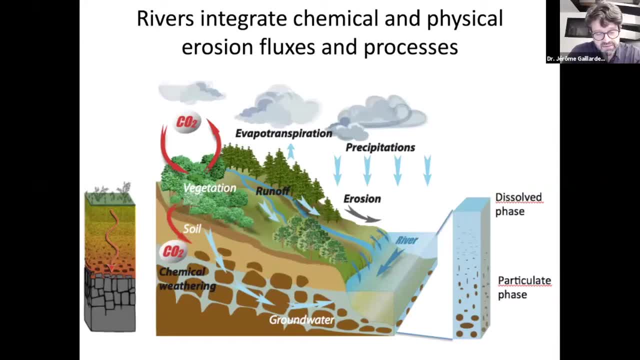 what is a critical zone? what are the limits of the definition? but basically, you should remind that the critical zone, which which lies between the rocks, the unwethered rocks of the lithosphere and the lower atmosphere, it's. it's a critical zone because it's one of the critical limits, interfaces of the planet, and it's a 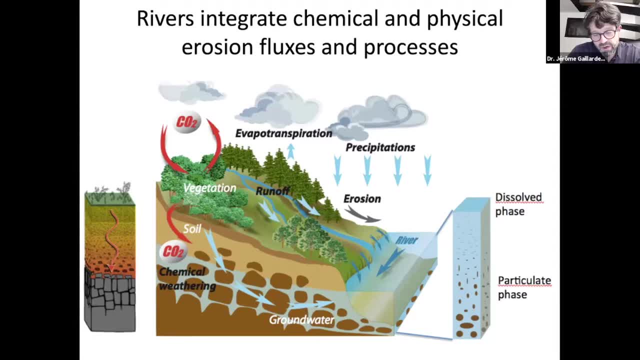 critical zone also because this is the where we live, where humans live, and this term, critical- was really well chosen because it's given, it's giving to this zone of interest a major philosophical and political role in in the global change that we live in. So the critical zone is a complex thing. it's. it's an, it's it's a multi compartment object. it is. 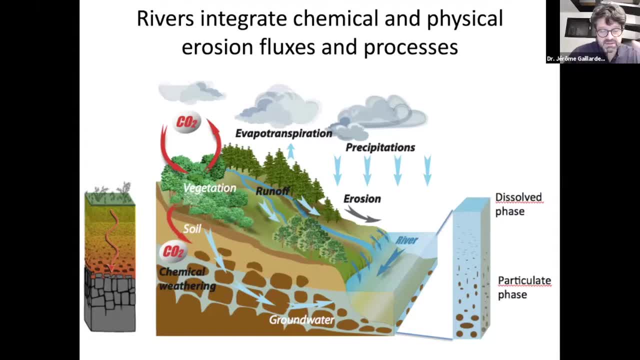 comprising the, the so-called ecosystems of vegetation. it's comprising the soil, the classical definition of soil. it's also fractures within in in which water is circulating. it's comprising the water, of course, and it's animated by a number of processes, and a couple of these. a couple of these processes are: 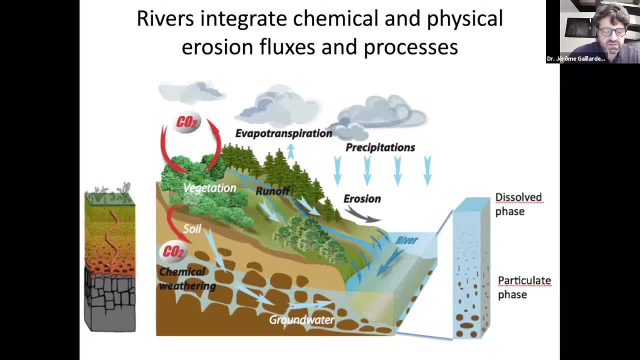 represented on this slide: precipitation, chemical weathering, which is a major process which is forming the critical zone, which is transforming the rocks into a porous, clay mineral zone at the surface of the planet. And so I'm using rivers as integrators of the critical zone, both as a source of 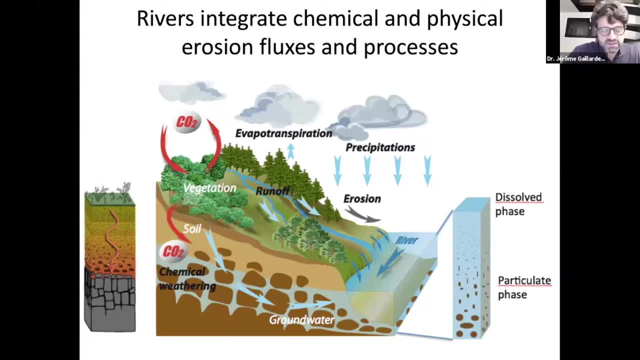 elements in in the rivers and the processes which are occurring in the critical zone. So rivers are nice because they are integrating over large surface areas, but of course they have the drawback that, depending on the scale that you're working at, you're not going into details. and of course, if you want, 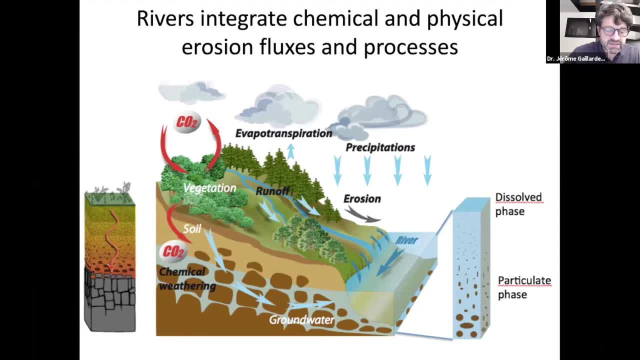 to go into details and to work on the scale. you're not going into details. and, of course, if you want to go into details and to study one single process, you you should go to a very small scale. but the scale I'm going to look at today is a very large scale, so I'm not going into the 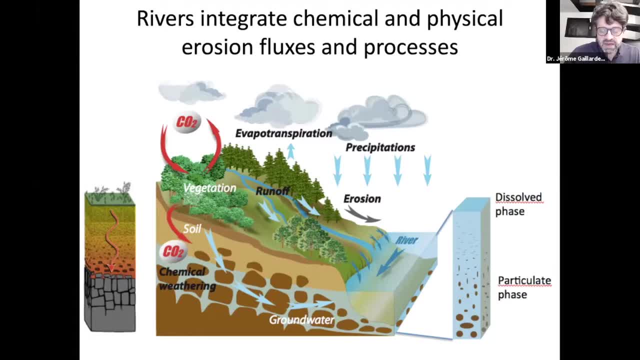 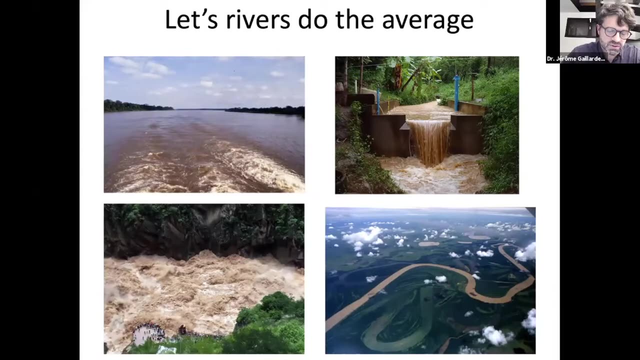 detailed process, but I'm using rivers as, as I said, integrators of these processes at the continental scale. So rivers do the average. this is a main advantage and this is why rivers have been used in the geochemical chart. Here is a couple of slides of rivers I particularly like, because I've been 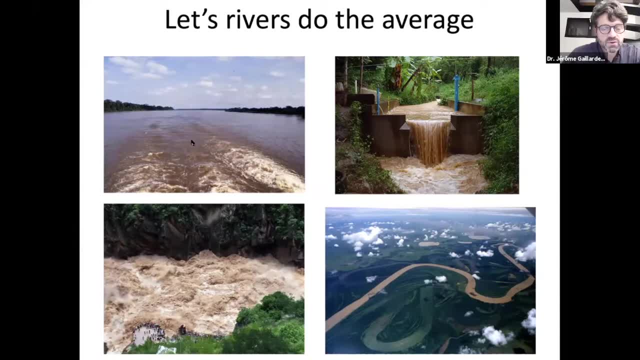 working on them. You have here the Congo River. Here a very different river which is flowing through the Himalaya, is the Chongyang or Yangtze River in China. This is the Amazon here at the bottom here, and here is a small catchment in. 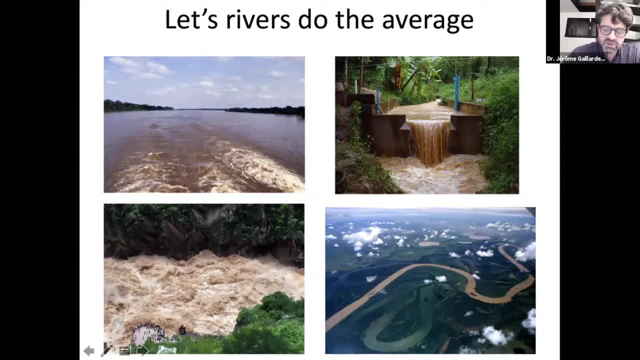 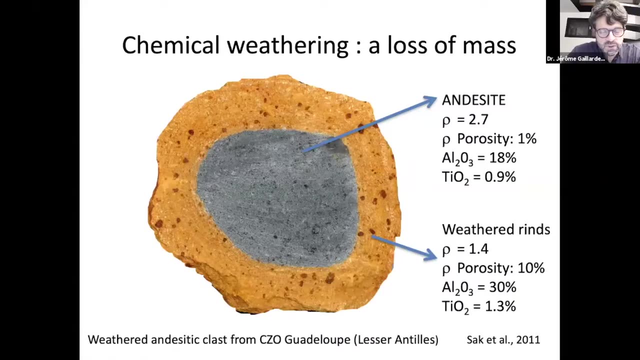 Laos, which is a Weipano catchment in Laos Which is characterized by very high physical erosion rates, as the picture is showing, with the ice suspended sediment. So the critical zone is formed by chemical weathering. So let me remind you what chemical weathering is in very 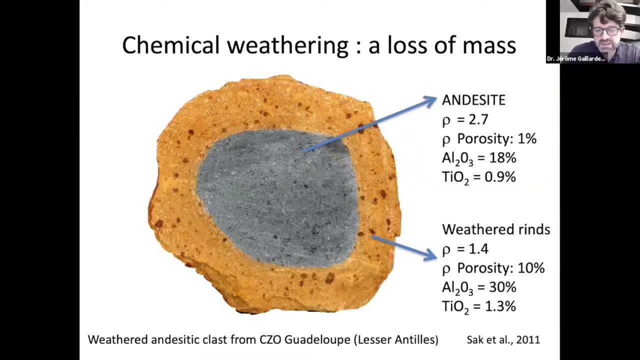 in a couple of words. So basically, chemical weathering is a loss of mass, and this slide is showing one of my preferred objects, Which is a volcanic bomb from from the lesser antis, and we've been working on on this rock quite a lot with my colleagues Peter Sack and Lin Ma from from El Pato. 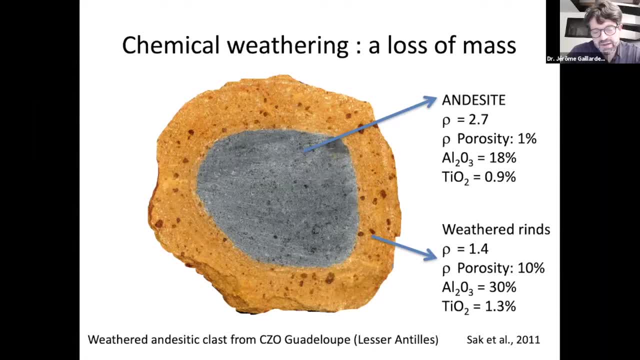 You can see on that slide, the, the center of the rock is made of an andesite which is not weathered. Okay, it's a, it's a, it's a typical andesite. The density is 2.7, the porosity is almost. 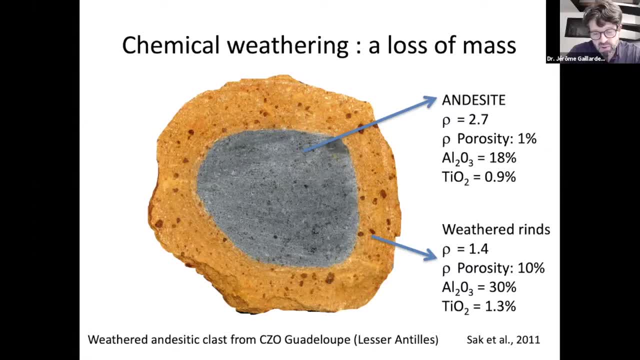 zero and the aluminum content is 18 percent. But when we, when we analyze and when we look at the, at the yellow external rind that you can see on that slide, it's totally different. It's it's it's derived from the transformation of the andesite, but it's totally different. 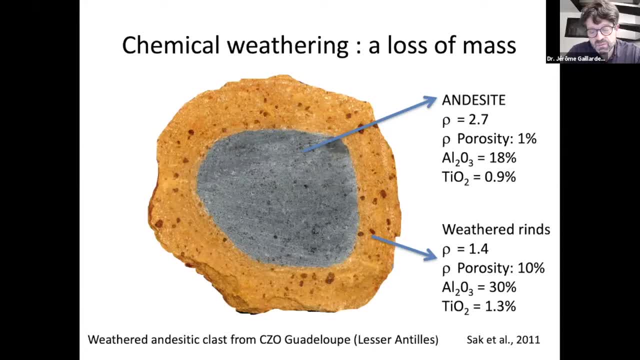 You see a density which is very low, you see a porosity which has increased a lot and you see the aluminum content, which is now 30 percent. So this simple example Show, shows you what chemical weathering is. it's a loss of mass between the the gray part. 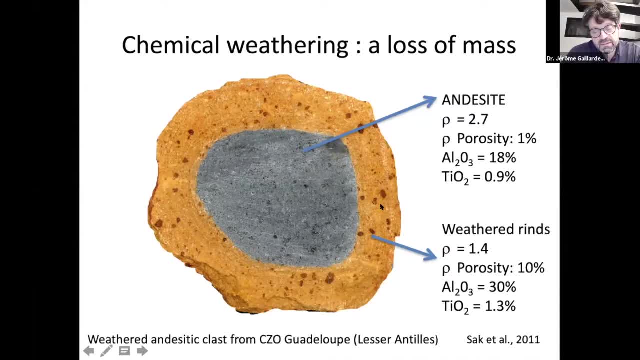 and the yellow part of the slide, Some elements which are essentially the cations- calcium, magnesium, sodium and potassium as left, and they have been transported by river, by the water which is continuously Weathering the, the rock and, of course, the material which is remaining as lost, a lot of. 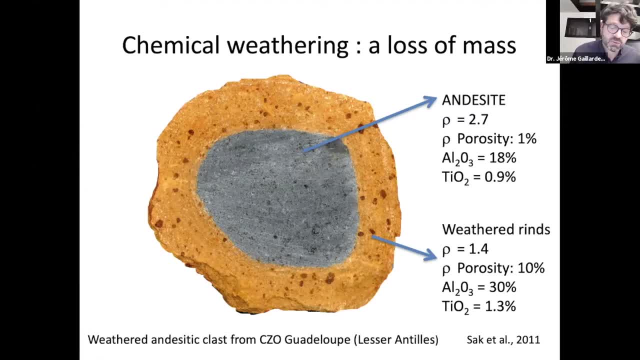 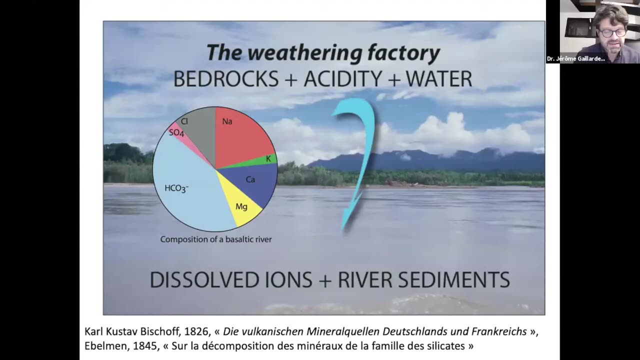 it Of of its initial mass and the elements which are remaining in the yellow part of the of the rock, and the most insoluble elements which are, for example, aluminum or titanium. And so where the cations? now, the cations have been transported by water. 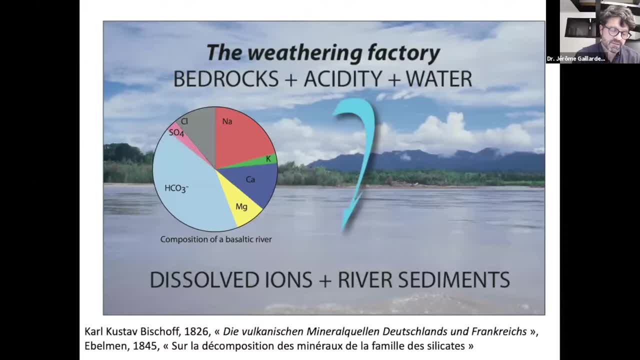 OK, they have left the system. and when we look very simply at the composition, the chemical composition of a basaltic river, here represented on this diagram, We do see that the major elements for most of the mass of the dissolved matter which is in in a litter of water is made of sodium, potassium, calcium and magnesium, which are 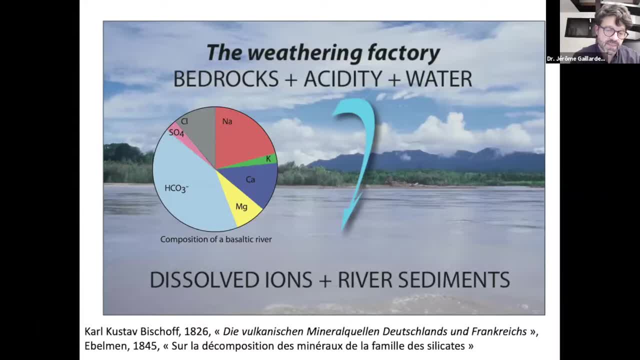 exactly the elements which have left the weathering, the weathered pellicule of the previous rock I have showed you. so, basically, the weathering process can be seen as a giant neutralization reaction. the, the, the acidity is the atmospheric CO2 and it's not water which is weathering. 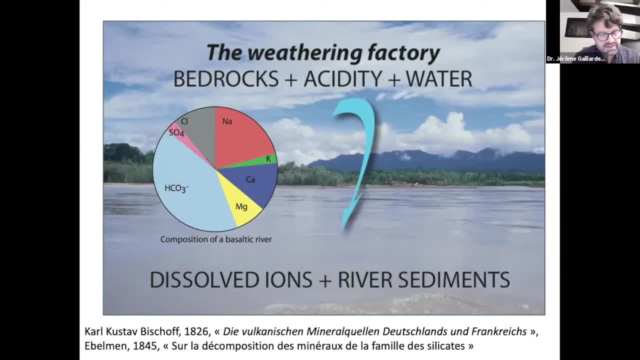 the rocks. it's the acidity containing water, and the acidity can can come from different sources and I'm going to show you different examples today, and so these acidity combined with water is transforming the rocks into something else, and this something else in the critical zone, and the critical zone is destroyed by 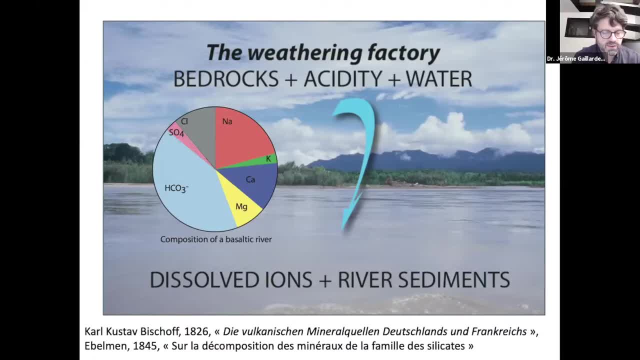 Physical erosion and ultimately, all the soluble and insoluble elements will get transported to the ocean by rivers. but so, by by studying rivers, we have an idea, we get information about these weathering processes at various scale and, in particular, at global scale. I would like to mention that this idea that chemical weathering is a neutralization reaction, 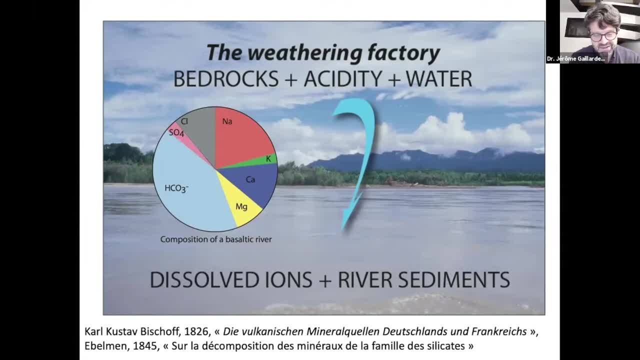 is not, Absolutely not, new. it's it's, and you can find very old articles, back in the middle of the 19th century, from this very famous German chemist, Gustav Bischoff, or this French mine engineer, Ebelman, which have initiated the idea or found the idea that that the 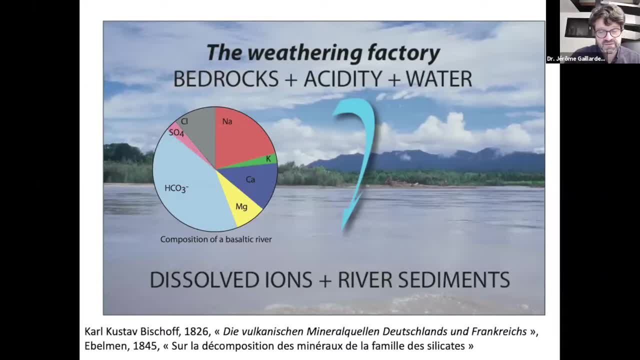 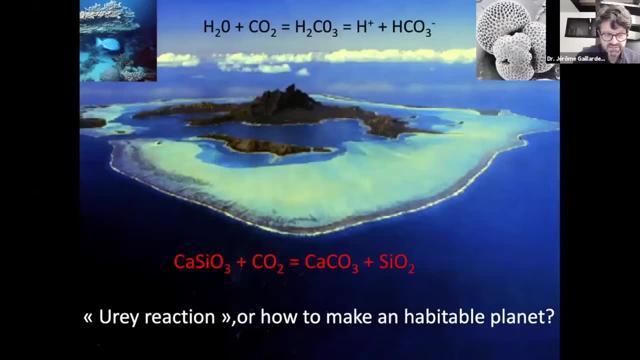 weathering was was a neutralization of of hair acidity By by the lithosphere, and so this mechanism of weathering is is very important for the planets because it is transport, transferring calcium, magnesium and over up cations from the continent to the ocean and these cations are precipitating into the ocean and, for example, 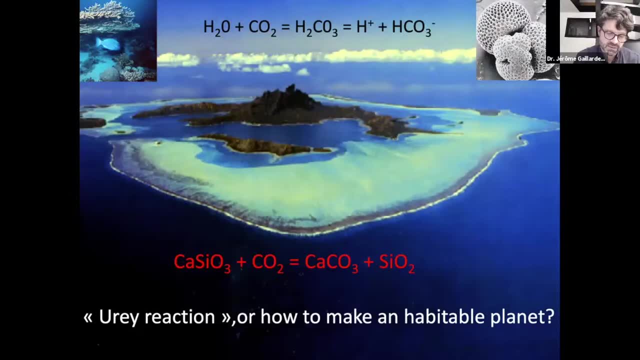 the best example is the formation of of carbonate in the ocean and- and this is I have showed you here- that is a so-called you air reaction, which is basically the reaction of carbonate In the ocean and- and this is I have showed you here- that is a so-called you air reaction. 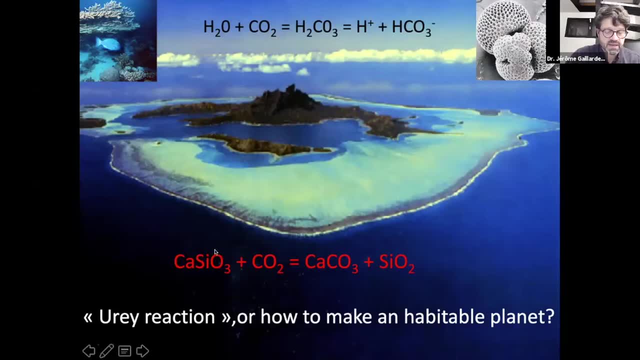 which is basically the reaction, That the reaction of calcium silicate, typical of the crust, of the continental crust, with the atmospheric CO2 will form, ultimately a calcium carbonate in the ocean, plus waste which is dissolved, silica. and this picture, which is a picture of a French atoll in the 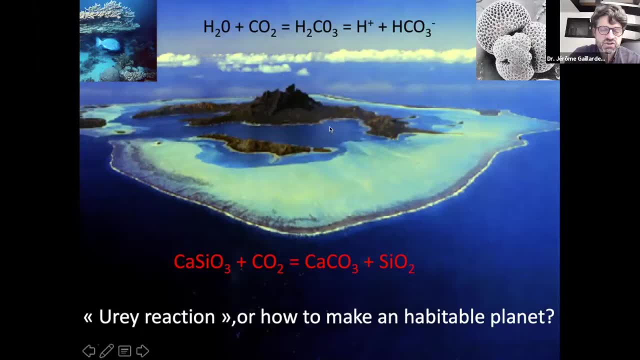 pacific ocean is. is is kind of a summarize of summarizing what is happening at the global scale. You have here in the center basaltic rocks. You have here in the center basaltic rocks which are being weathered. the calcium is moved. 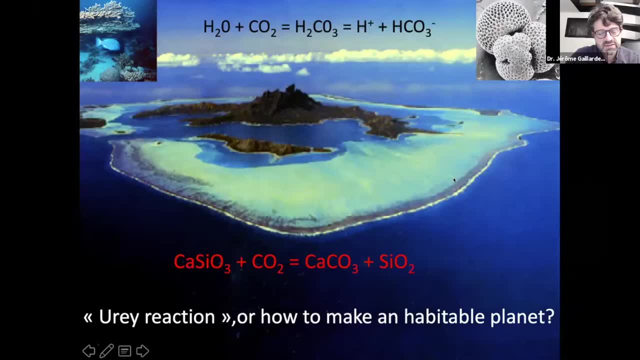 from the land to the ocean and it's precipitated in the form of carbonate. but in the meantime, the CO2 which has been used to weather the basalt is now sequestered in the carbonate. So this reaction has allowed the planet earth to lower its initial atmospheric CO2, which 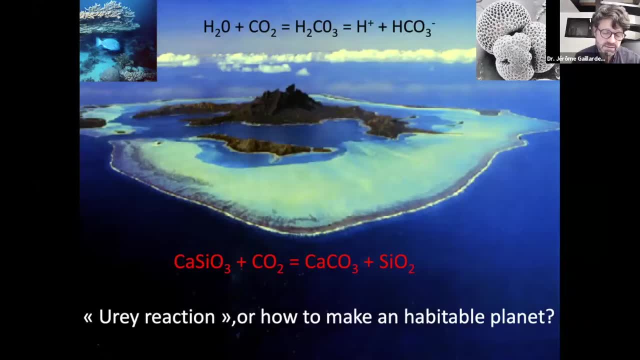 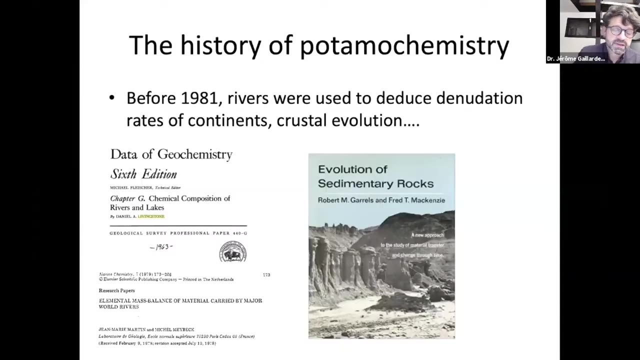 was very high and close to what it is still now on venus or mars, to something which is very low and constant, compatible with a temperature, a climate and a temperature which is good for life and the development of life. So I'd like to show you a couple of slide on the history of potamo chemistry, if I, if 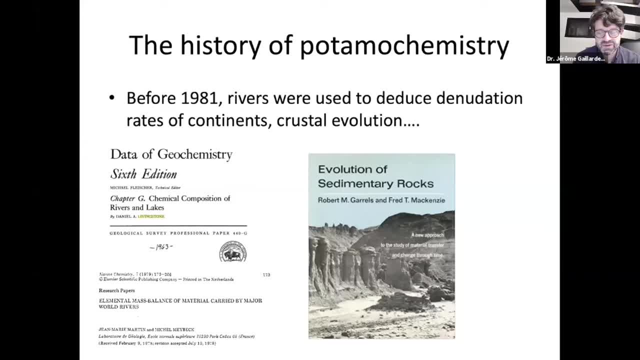 I can, if I, if I can say so. potamo in greek means the river, and the potamo chemistry is the chemistry of rivers, and it's very interesting when you start to look at At When people started to publish data on river chemistry. it's, it's it. you can go very far. 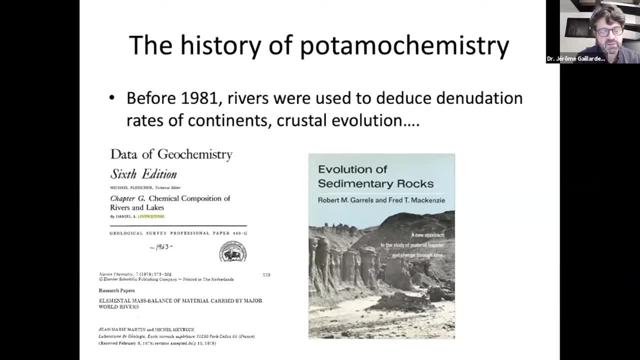 in the in the past and some of the seminal papers have been published by a guy named livingstone in the us in 1963 and and and maybe in paris, and martin published a number of important papers where they, they, they started to to, to summarize and to put together data: 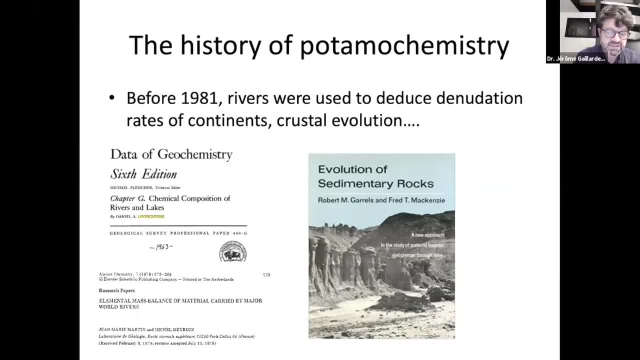 on river chemistry. And of course there is a seminal book by garell's and mackenzie, which is 72- 1972, which is using the river chemistry database to infer information about the denudation rates of continents. so before 1981, essentially river data were used to infer information about the denudation. 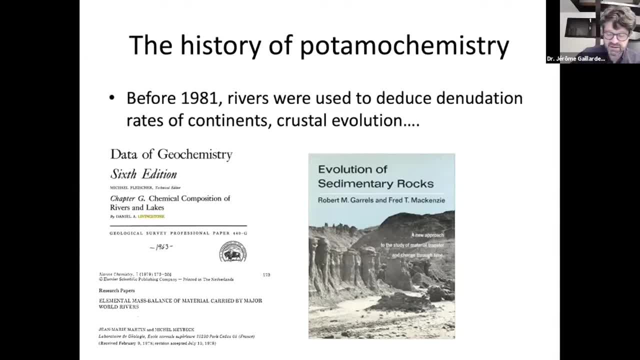 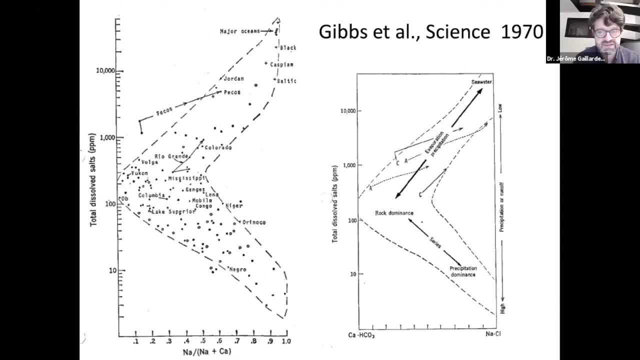 rates of continents or the crystal evolution, this kind of thing. And there is one Significant paper which is very well known by gibbs at all in science in 1970, 70, which is trying to determine the control of a river dissolved, the river, chemistry as a function. 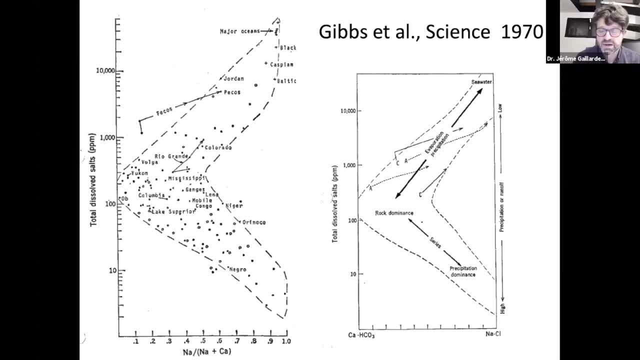 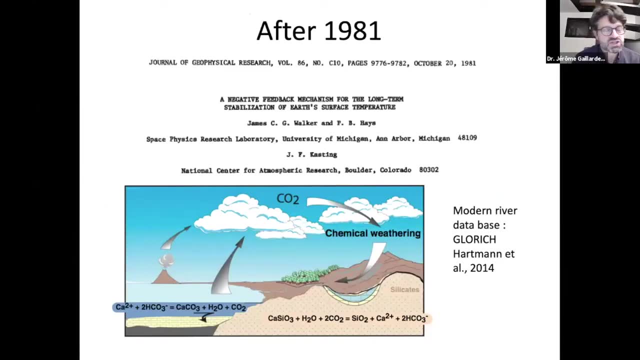 of evaporation, lithology, precipitation, etc. this is a very important paper but something happened in 1981, which is the location of very famous In The paper in the chemical community, which is the paper by walker at all, which is basically assuming that the earth climate is stabilized by your feedback, in which silicate weathering 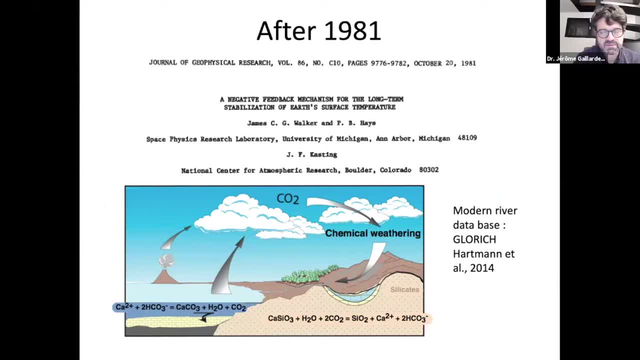 Is acts as as as a feedback mechanism, as a buffering mechanism. basically, the idea of the paper is to say that if you have a lot of co2 in the atmosphere, temperature is going is going to increase And then this weathering of silicate is going to produce more calcium to the ocean and you 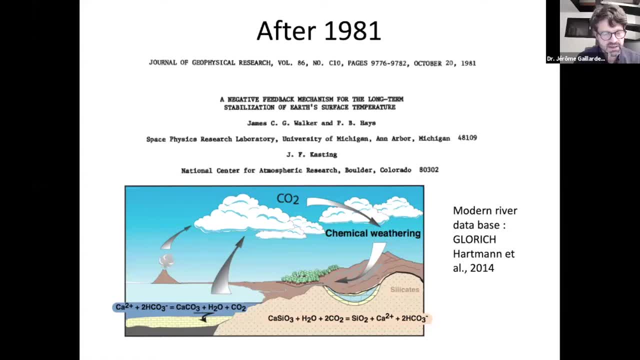 will precipitate more carbonate into the ocean, and then you have a mechanism which is able to Stabilize the earth climate. this, this was a very important paper and this is still a very important paper, but my point today is to show you that this paper has triggered 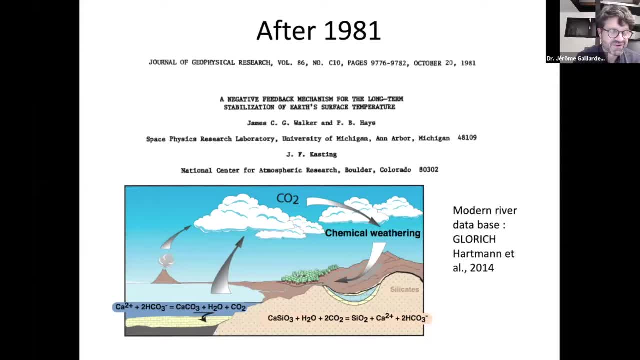 a total Phenomenal Increase On The number of paper on the rivers, because suddenly people walking on rivers realize that the data that they were measuring and accumulating Could be very useful to test this thermostat hypothesis. the paper of walker and at all. 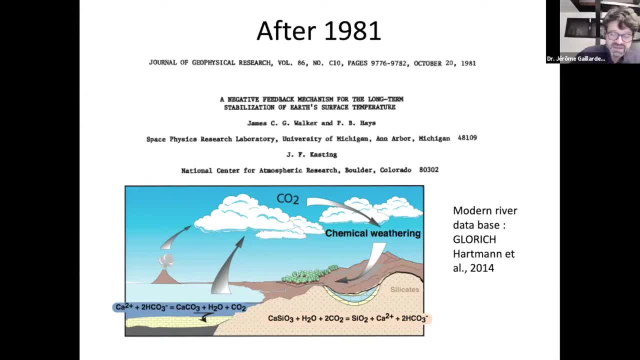 published in nineteen ninety one, So after nineteen, eighteen, ninety, eighty one, the, the, the introduction of the of the paper Of the Dealing with the geochemistry of river, of rivers, mentioned the fact that silicate weathering was, was a sink of co2, and and so by studying rivers, you would eventually be able to calculate. 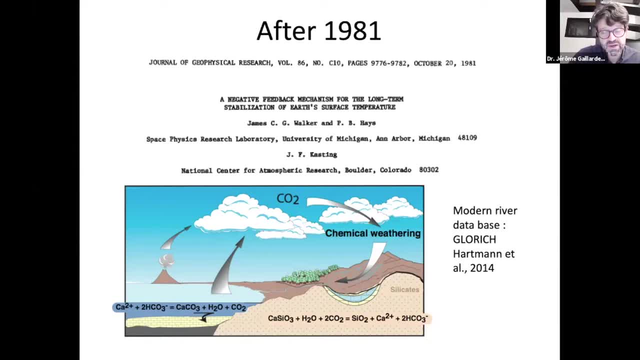 the rates of suit of co2 consumption and then to to build models and to test the hypothesis which was proposed by Walker at all. So, so, So. So, today we have now big that the buzz, and I I would like to mention the last update. 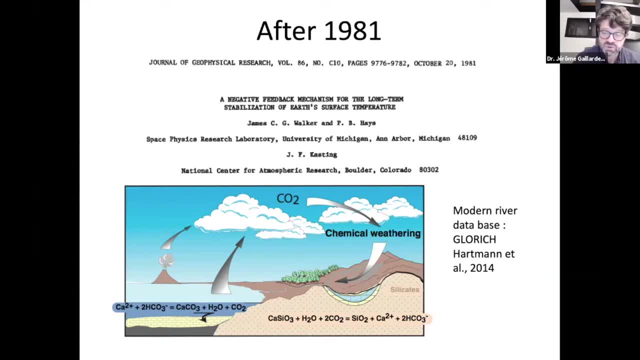 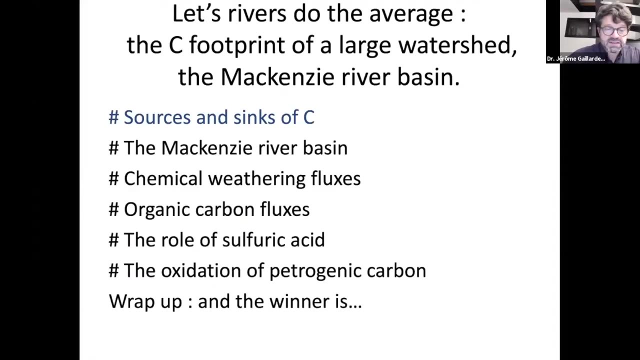 on on modern river geochemistry, which which is a database which was constructed by Jens Ackmann from Hamburg in Europe, and it was published in two thousand fourteen and which is called Glourish OK. so today I would like to take one example of how we can use rivers. 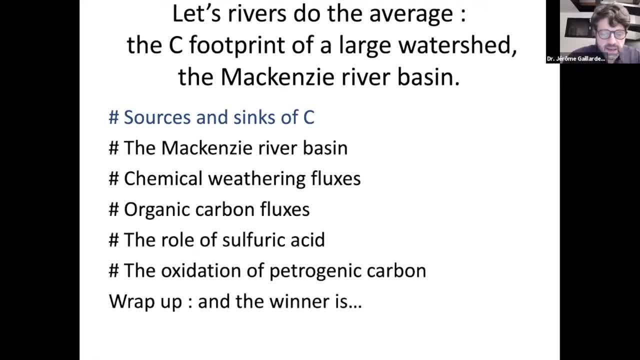 and And To integrate Critical zone processes. and the question which I'm interested in today is to make a complete mass budget Of carbon at a very large scale and, in and with the application of the Mackenzie River Basin, very few basin, if not, maybe only two. 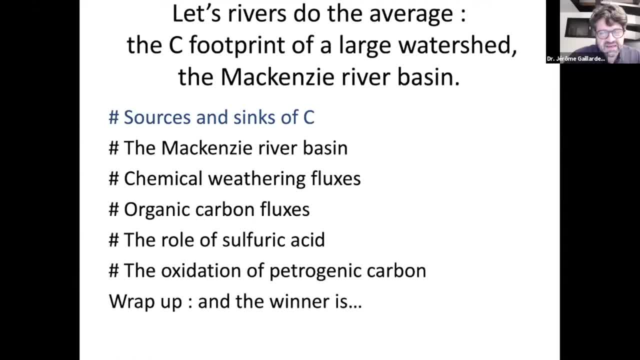 River basin, as has been investigated by, by the way I'm I'm going to show you tonight. So I mean by by this investigation, I mean to make The list, All the list of the list of the, all the processes which are sources and sinks of carbon within. 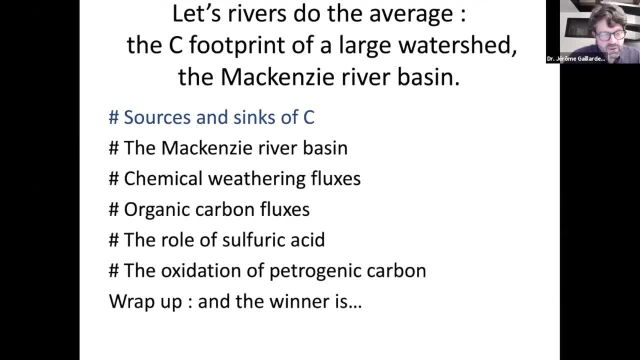 the watershed and to calculate at the end what is the net result. OK, so basically I'm going to again to test whether the Walker at all I bought is this works, In other words, if The earth Surface Is a way to consume CO2 from the atmosphere. 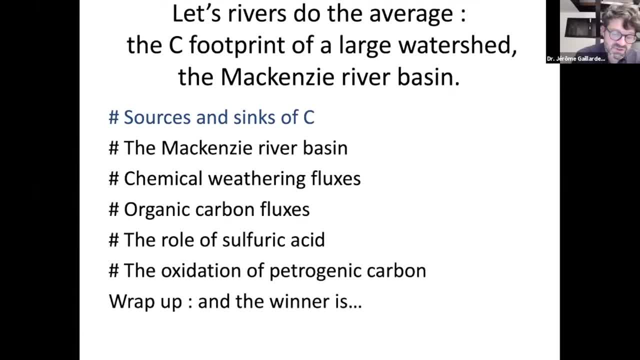 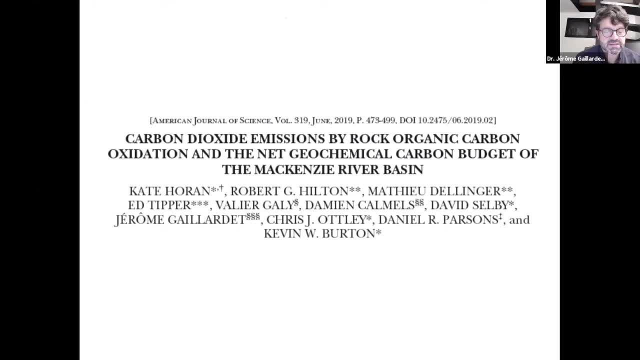 OK, And so this corresponds to a paper that we have published the very last year or two years ago. The first author is Kate Oran, from from Durham, and this paper is associating a number of friends and colleagues that you can see here, Bob Hilton. 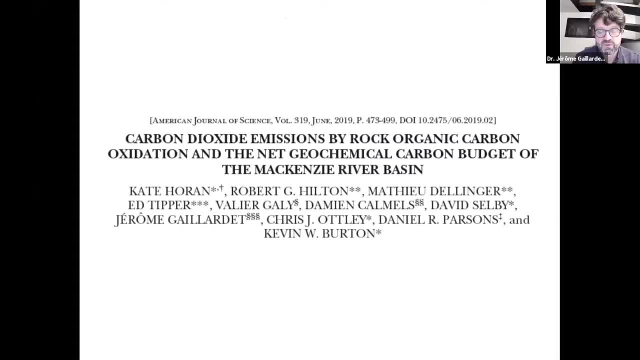 Mathieu Delanger, Ed Tipper, Valle Galli From Woods Hole, Damien Calmel From Orsay University And others, And so this is a big paper which is making a synthesis of, in the catchment of the Mackenzie River Basin, of the net CO2 consumption. 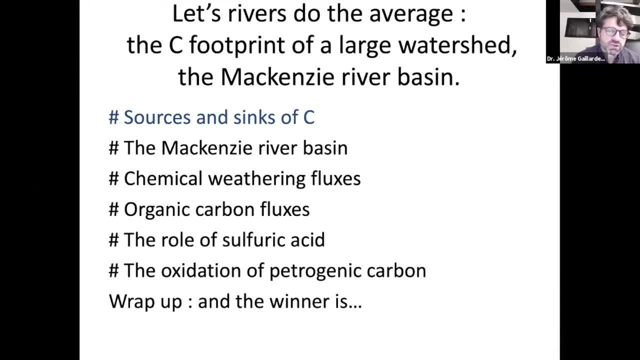 So Now, To show you what are the sources and the sinks of carbon in theory, I would like to talk a little bit about the Mackenzie River Basin. I will show you How we calculated the chemical weathering fluxes, So the inorganic 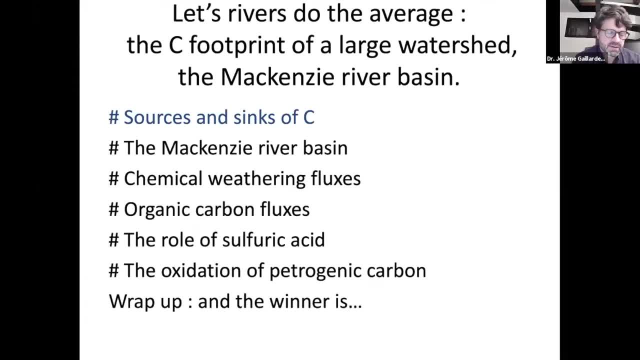 Chemical weathering fluxes. I will then Turn to the organic carbon fluxes. I will Insist on the role of sulfuric acid, Which is a new discovery in the field of river geochemistry and which is totally changing the The vision that 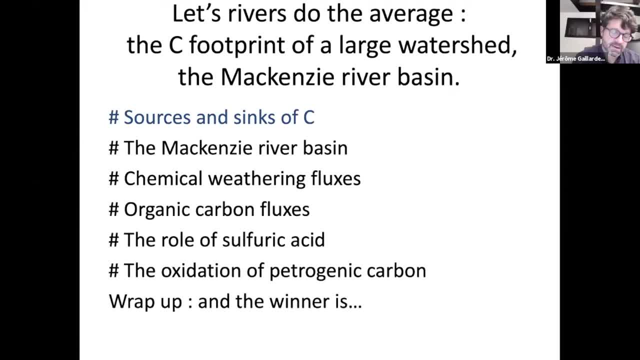 Walker Add In 1981. And I would talk about the oxidation of petrogenic carbon, And then I will work, Wrap up Everything And I will give you The name Of the winner. I mean, Is it? 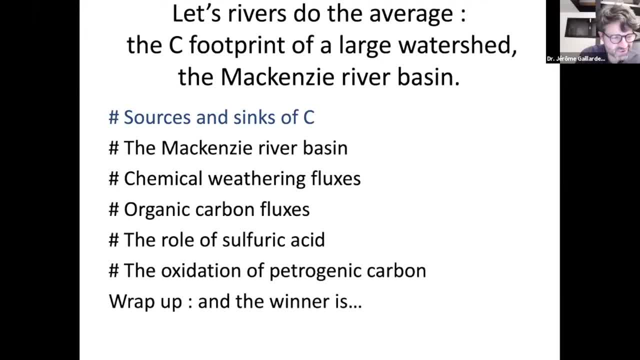 Is the Mackenzie River A source Of CO2 to the atmosphere, Or Is the Mackenzie River Basin As a sink Of CO2. At the end? So A little bit Of, A little bit Of. 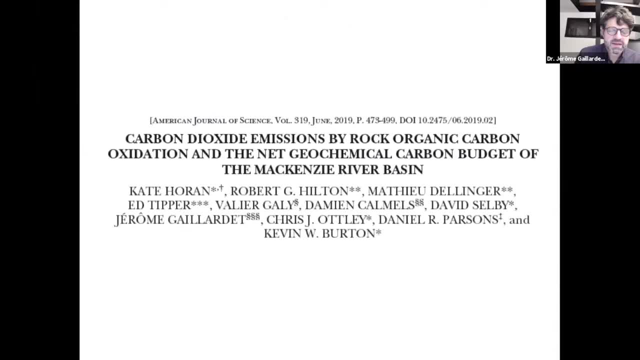 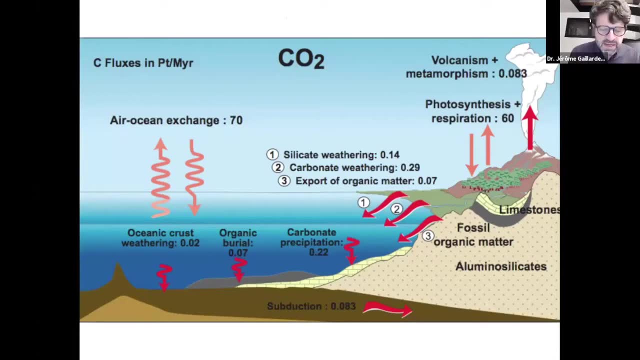 Of, Of, Of Of. Now A little bit, A little bit Of theory. So this is a slide showing you the different coven cycles. So basically, I don't want to spend too much time on that, but there are. 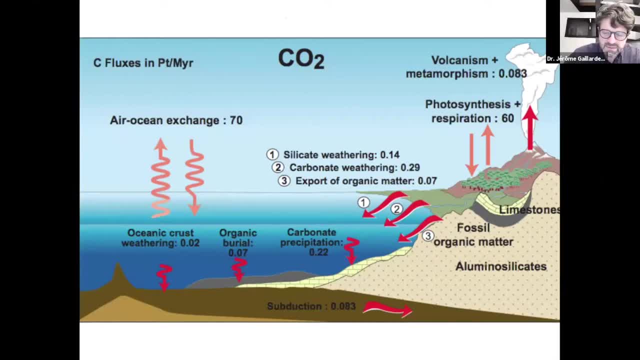 Many, Many common cycles: And And, And And so. So short Common cycle is the cycles We, the cycle of carbon, Which is Associated, Associating for the synthesis and the respiration. Okay, it's a very short term, pretty much equilibrated, and so I'm not going to talk too much about. 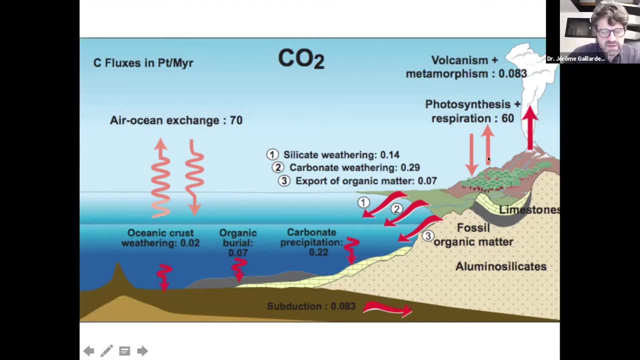 photosynthesis and respiration in the Mackenzie River Basin, because I'm considering that these very short-term fluxes are equilibrated. But on a longer time scale, a number of processes are consuming CO2 from the atmosphere and sequestrating it into the ocean. This is silicate. 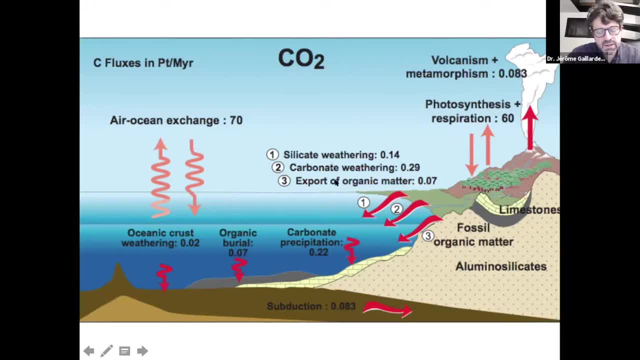 weathering. this is carbonate weathering and this is the export of organic matter that some people call a weathering of organic matter, which I think is not a proper term. And all these fluxes, the red arrows here- correspond to carbon, which is transferred from the atmosphere to the ocean. 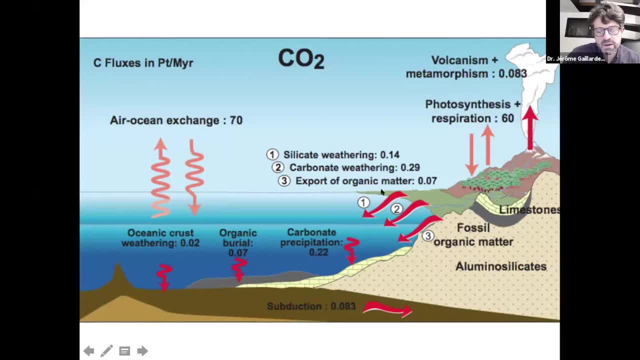 So if I want to make a complete mass budget of what is happening on a catchment at the surface of the crop- the compare with carbon to carbon across the atmosphere Scale over a micrometer planet- I must take into account all these fluxes And this is what I am going to do today. So just 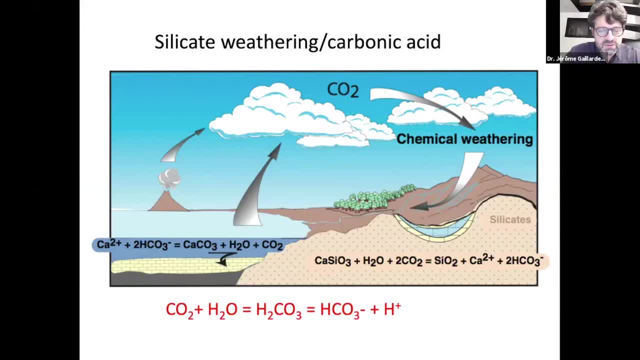 a quick reminder of why silicate weathering is a sink of CO2.. I have already gave you a couple of words on that, So this is a slide showing the chemical reactions associated with the weathering of silicate: the calcium silicate here on land and the precipitation of carbonate into the ocean. 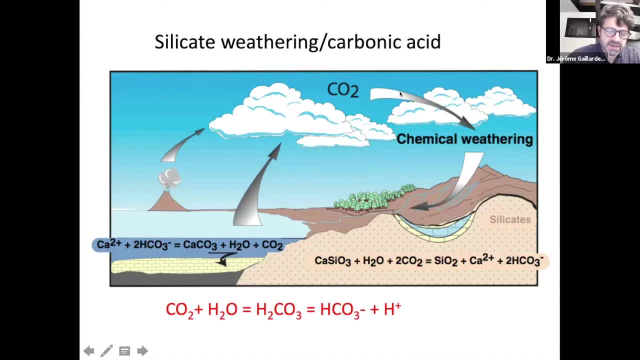 So, over the time scale that is characteristic of this carbon cycle, and we don't exactly know, but let's say half a million year, the typical time scale of that process is half of a million year- You consume CO2 from the atmosphere because you see, you do see that when you 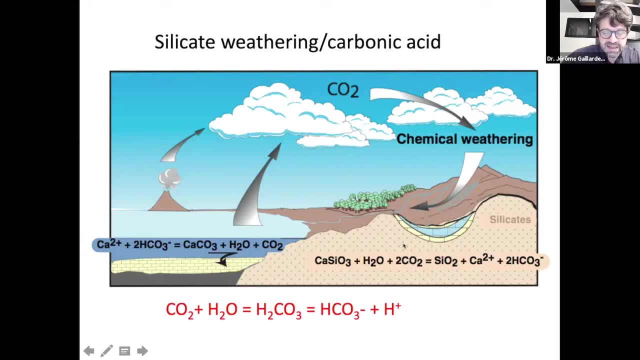 want to have a carbon cycle, you have to have a carbon cycle. When you want to have a carbon cycle, you have to have a carbon cycle. When you want to have a carbon cycle, you have to have a carbon cycle. Whether one mole of calcium silicate on land, you consume two mole of CO2, but when you precipitate, 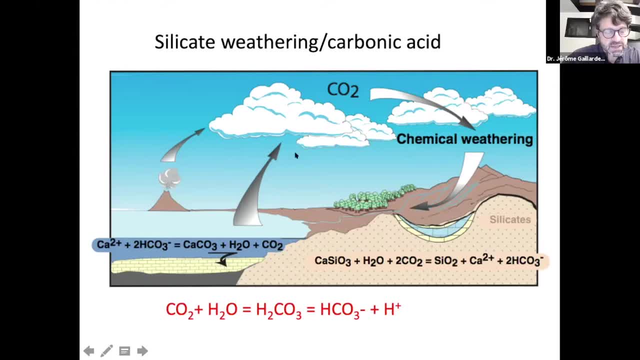 calcium in the ocean, you remove one mole of CO2 into the system- I mean into the ocean plus atmosphere system. So the net result is the transfer of one mole of carbon from the atmosphere to the limestones here, And this is a long-term process by which probably the has purified its. 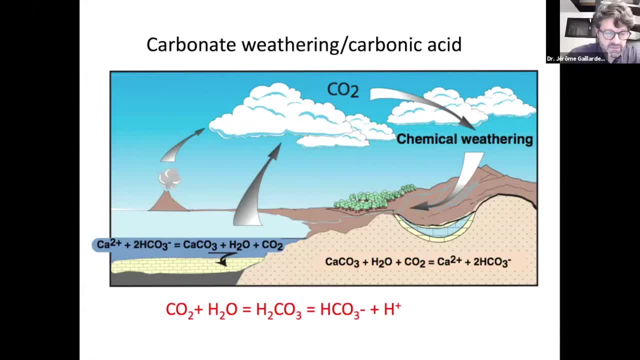 atmosphere in CO2.. And this is a long-term process by which probably the has purified its atmosphere in CO2.. And this is a long-term process by which probably the has purified its atmosphere in CO2.. If you consume carbonate weathering, you consume CO2 from the atmosphere to make this reaction here. 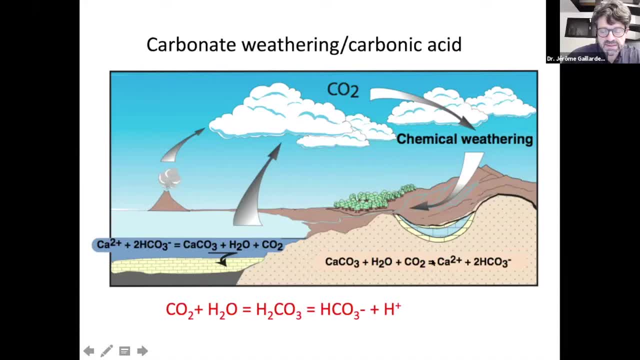 One mole of common calcium carbonate is reacting with one mole of CO2, but when common calcium carbonate is precipitating into the ocean, it's exactly the reverse reaction, And then you remove the CO2 that you have consumed. So if you think about long time scale, 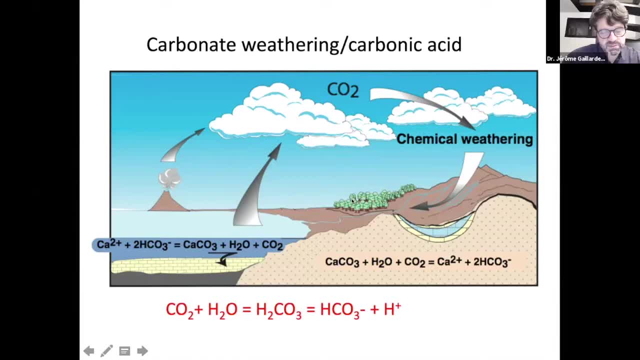 such as half a million year, which is a typical time scale of silicate weathering cycle. you are tempted to say that carbonate weathering is not a source of a sink- sorry- of CO2 from the atmosphere, that actually this is not really true, because at smaller time scale and typical, for example, typically 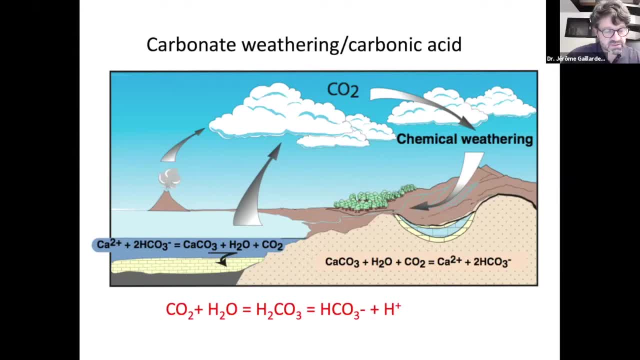 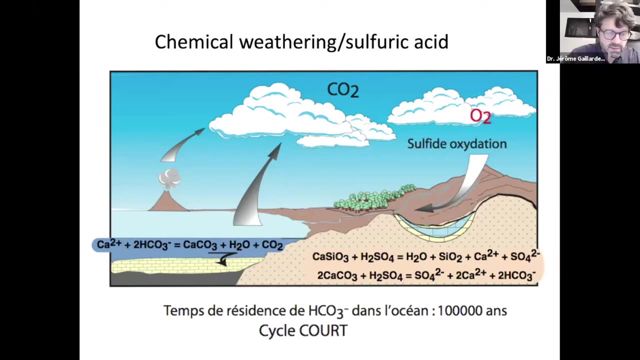 is a timescale which humans are perturbating. the system component counts. calcium carbonate is going to to matter, and when you weather. in addition, when you weather calcium carbonate, not with carbonic acid, which is a co2 from the atmosphere, but with another source of acidity, which is provided by the oxidation of sulfide, but that produce sulfuric 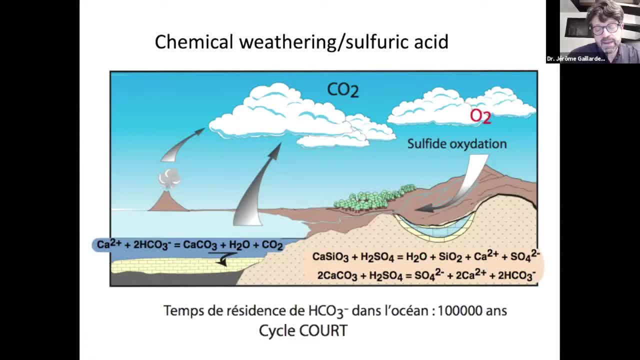 acid, then you will have another, a very different situation, because you do not consume co2 when you weather the limestone on on terrestrial surfaces, but you release co2 in the ocean when you precipitate the calcium carbonate. so um, and and has been published by a number of of authors over 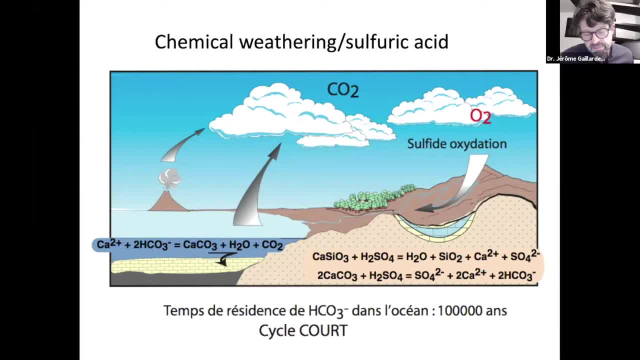 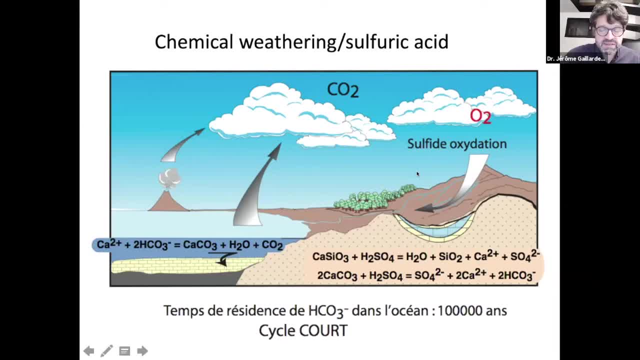 whether the continental crust, but basically, if you use another source of acidity than carbonic acid, then you will remove co2 in the atmosphere over a certain period of time, of course, if you go at very long time scale, the, the sulfate which is added to the ocean by the 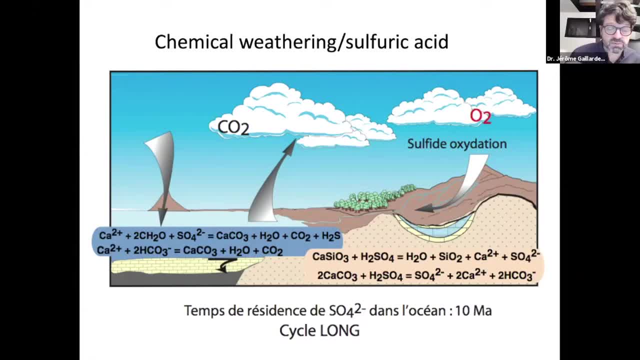 weathering of limestone by sulfuric acid is going to be reduced in sulfide and then you will have exactly the reverse reaction that the one you, you had on land and so over very long time scale, which are great, higher than the resistance time of sulfate in the ocean, so typically 10 million. 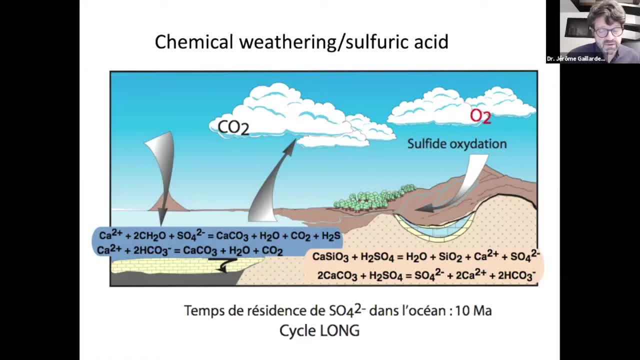 years. the chemical weathering of limestone by sulfuric acid is not a source or a or a sink of co2 from the atmosphere, because the two the equations are are balanced, but on transient time. it's important to realize that when carbonate weathering is made by the you, by by using 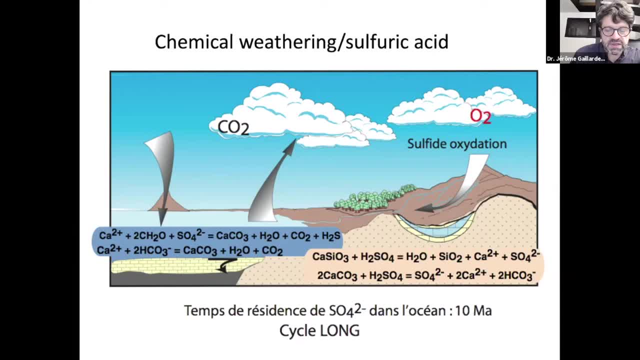 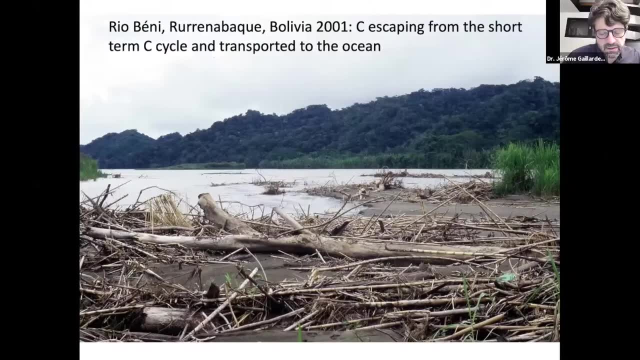 sulfuric acid. it's a source of co2 to the atmosphere. so these sites were about the, let's say, inorganic cycle. but there is another cycle which is organic now, which is represented on that slide. this is a slide of the benny river in the andes and you, you do see that, that on the 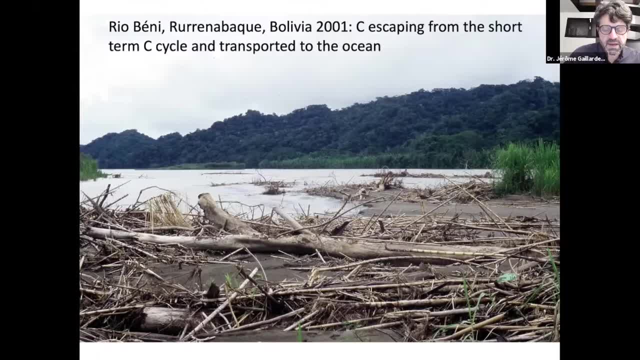 beach of the end of the benny river, you do see branches and and residue of organic matter which has been physically eroded from the landscape and is going to be transferred to the ocean. so eventually, this carbon is going to be burial, buried and is going to be- uh, to represent a net sink of co2- co2 which has organic matter. 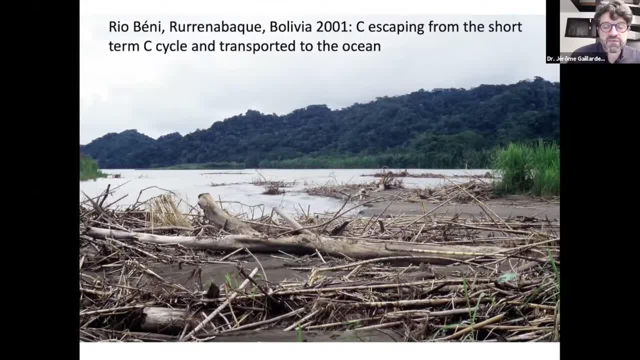 containing carbon and this organic matter has a scale of the carbon that is being kept from the roman romanization of organic matter in the in the top side. so organic burial is a is a very important process which is sequestrating co2 and but of 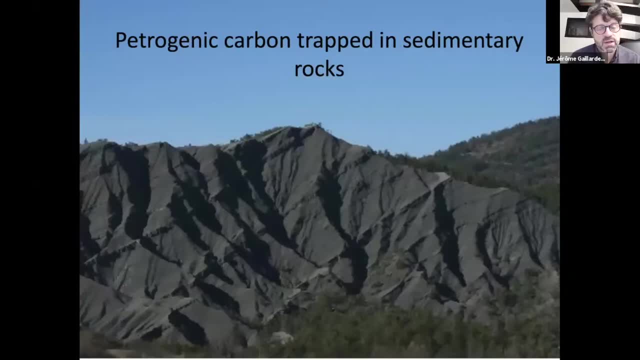 course, you also have the reverse reaction, which is the oxidation of carbon, of heterogenic carbon, of fossil carbon trapped in sedimentary rocks, and this slide is showing a typical image. um, this is a very particular image that you can see in a paper by jim raymond uh. 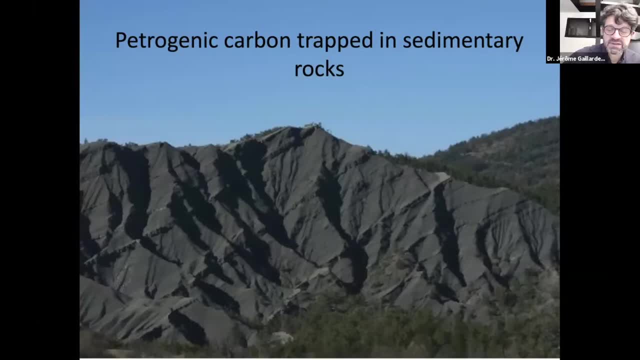 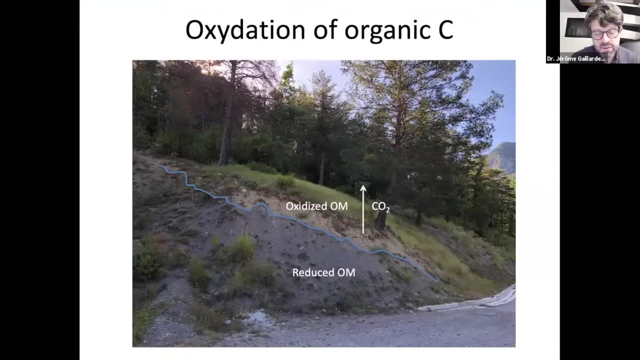 the rock is being contained, formed by organic rich sedimentary rocks, and at the surface we don't see that on the slide, um, but but if you go in, emotional rocks exposed to the, to the oxygen of the atmosphere, of the modern atmosphere, are going to be oxidized, just because the organic matter of the rock is very reactive in contact with 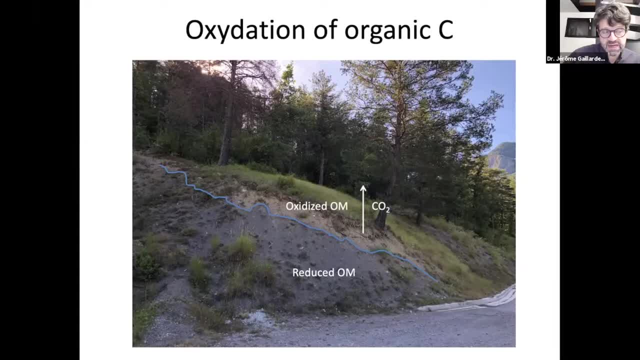 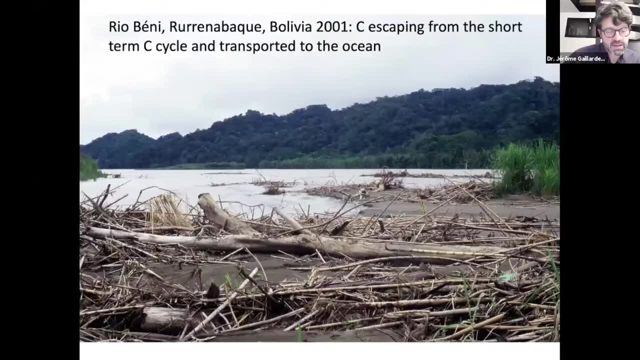 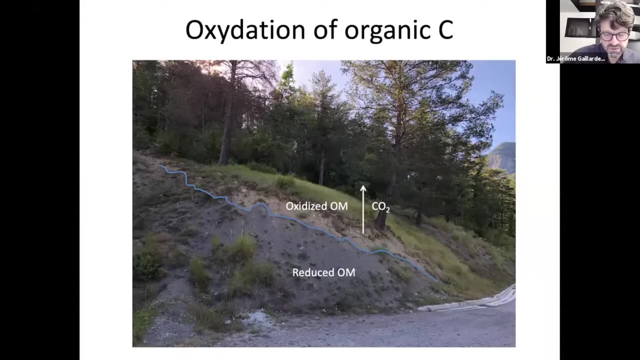 So this is a reaction which is producing CO2 to the atmosphere. So it's a counter reaction of the previous one. The burial of organic matter is compensated by the oxidation of fossil organic matter from terrestrial surfaces. So you do see that it's a very complicated situation. 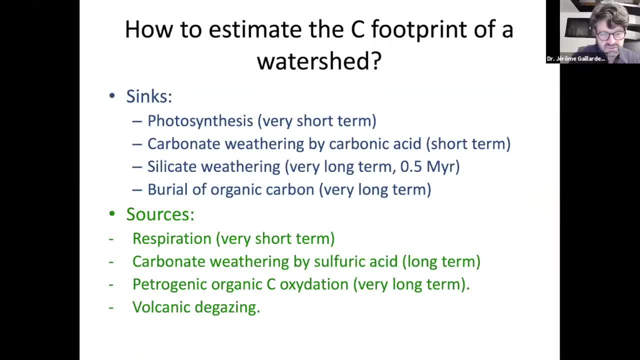 And if you want to make a complete mass budget, you have to take all this into account. So you have to take into account the sinks. photosynthesis- I'm not going into photosynthesis processes today because, as I said, it's a very short term process. 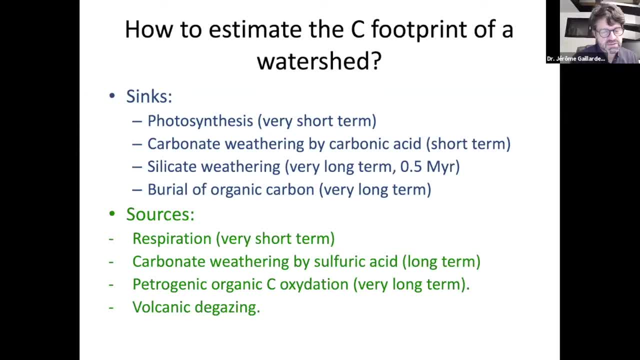 But carbonate weathering by carbonic acid should be considered. Silicate weathering should be considered. The burial of organic carbon should be considered. These are the sinks of CO2 from the atmosphere. But you also have sources: Carbonate weathering by sulfuric acid. 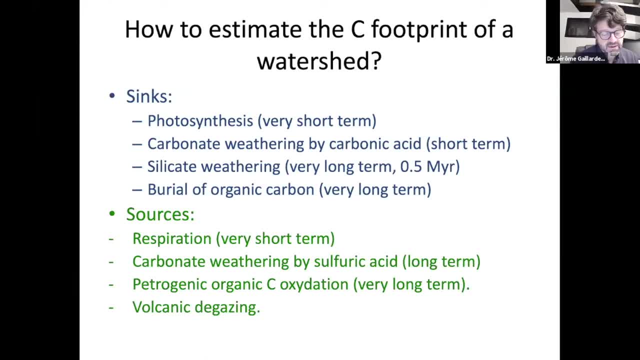 I just showed you that this is a source of CO2 to the atmosphere. You need to take into account the oxidation of the petrogenic carbon present in the rocks, which is producing CO2 to the atmosphere And, eventually, if you have volcanoes on your watershed. 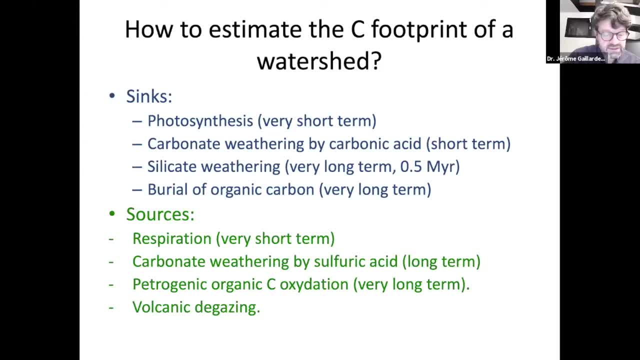 you should take volcanic degassing into account. This is not the case in the Mackenzie River Basin. Okay, so I'm going to show you how we solved this problem in the Mackenzie. I'm not going into the details of all these processes. 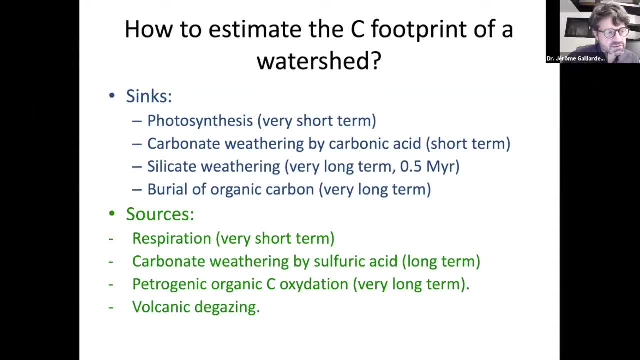 and how we did exactly to get the CO2 consumption or CO2 emission numbers- But I'm going to screen the different processes here- and how is it possible to use river chemistry to get the numbers of CO2 consumption and CO2 emissions for, at the end, calculating the net CO2 exchange? 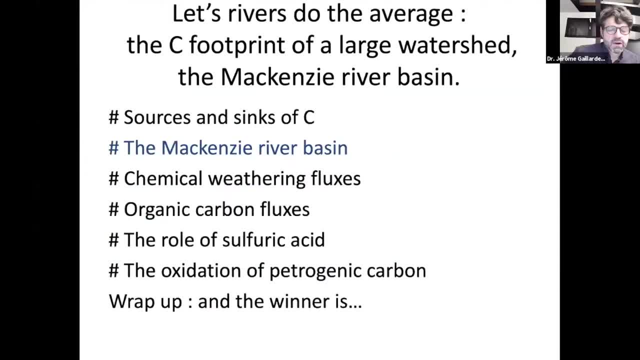 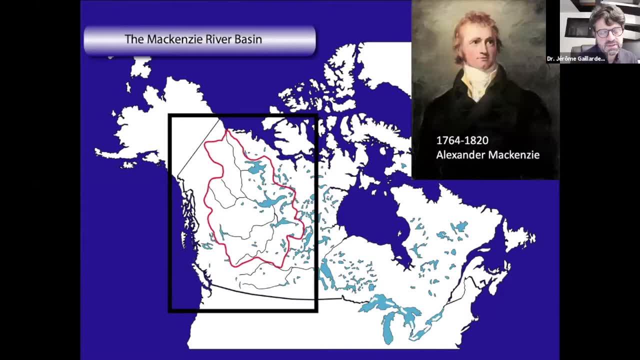 in the atmosphere and the Earth's surface. Okay, so let me talk very, very briefly about the Mackenzie River Basin. So it's a nice, very nice catchment watershed in the northern part of Northern America. It's taken its name from the Alexander Mackenzie. 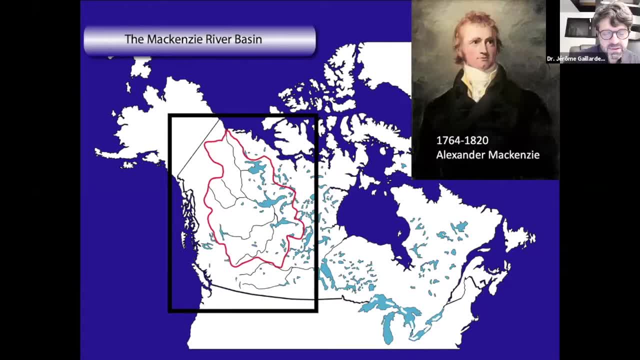 which discovered or first described, the Western guy which first described the basin. It's a pristine basin, So you're not worried. You don't have to worry too much about human activities in the Mackenzie River Basin, which is not true, I agree, for gas exploitation. 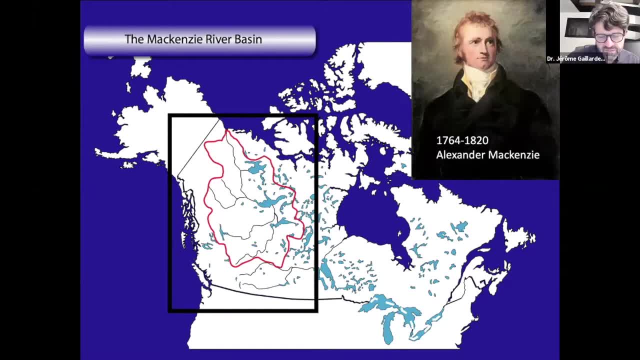 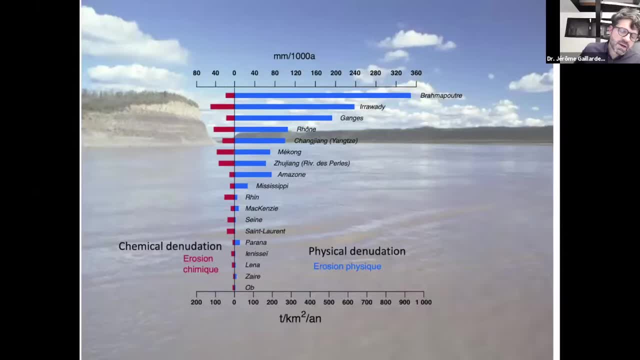 but you don't have a lot of pollution in the river that you should correct for It's a relatively pristine catchment. In terms of physical denudation and chemical denudation, the Mackenzie River is not very impressive. It doesn't have very high. 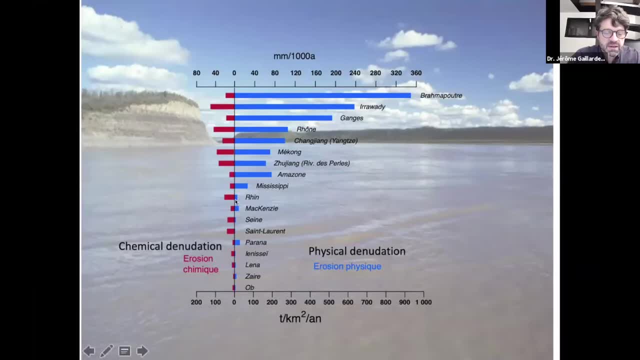 very high fluxes of denudation. It's here. It's very, very different, of course, from the rivers draining the mountains of Asia, but it's not totally. it's significant And in particular, it is significant for the inputs of sediments to the Arctic Ocean. 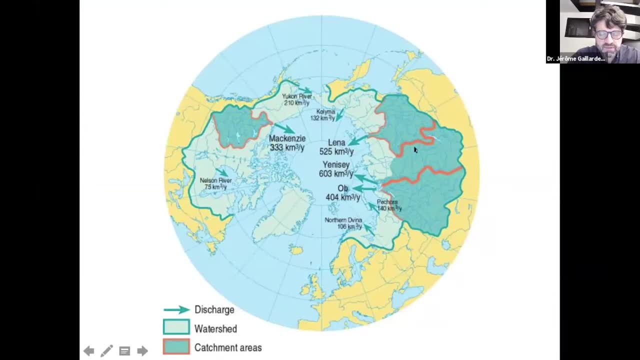 So this is a map showing the water discharge of the different rivers draining to the Arctic Ocean. So the Mackenzie has a significant discharge in comparison to the Russian rivers here. But if I were to look at the suspended sediments and the physical erosion, 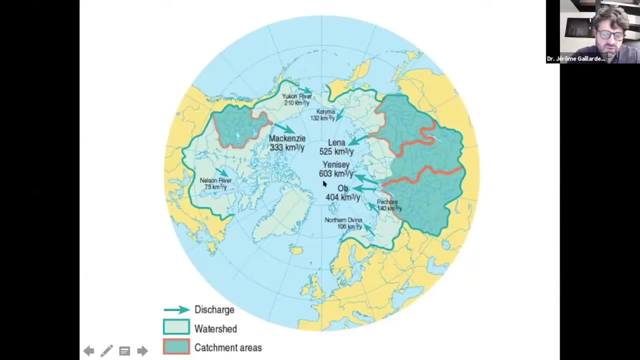 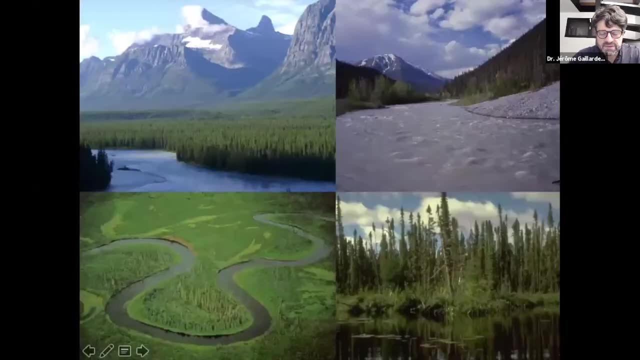 the Mackenzie is the main contributor to the Arctic Ocean in terms of sediments. So this is some pictures of the Mackenzie River Basin: the rocky mountains- Here you can see the water You can see here, with rivers usually very loaded in suspended sediments. 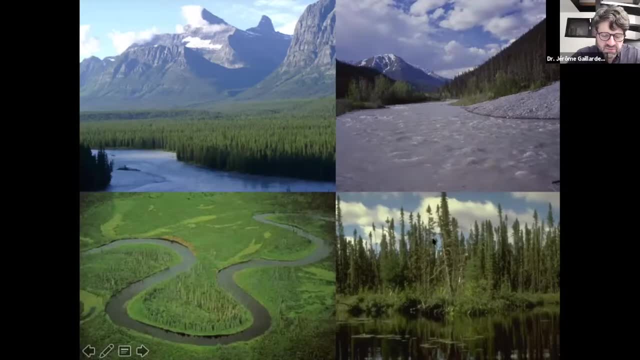 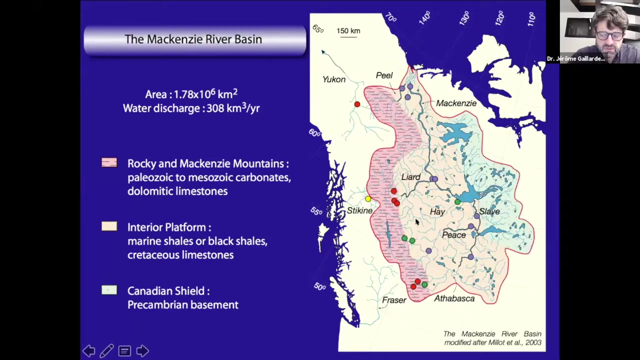 derived from the glaciers, And this is pictures from the lowlands, with beautiful and typical meandering rivers and swampy areas. In terms of geology and relief, the Mackenzie River Basin is divided into three main parts At the east. here you have a region which is a slave. 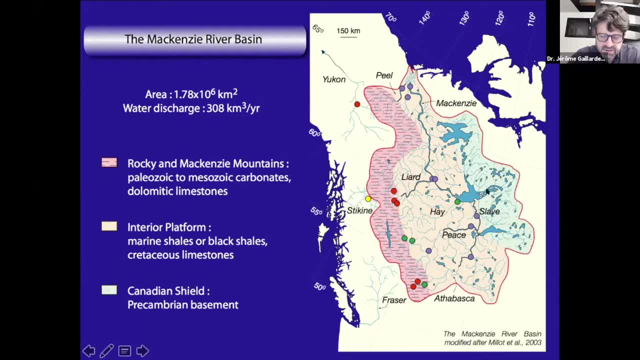 province is a granitic, very old and quiescent region, not very much contributing in terms of water to the river. Here you have totally, at the west, the Mackenzie and rocky mountains, which are essentially made of paleozoic and mesozoic carbonates, shells and dolomites. 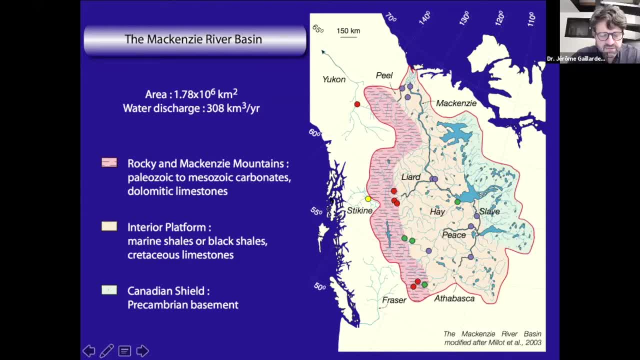 And in between you have the interior platform, which is very flat, very swampy, and which is constituted mainly of marine shells and black shells from the Cretaceous, And so the points here are the data that we have collected, So it's a very long story. 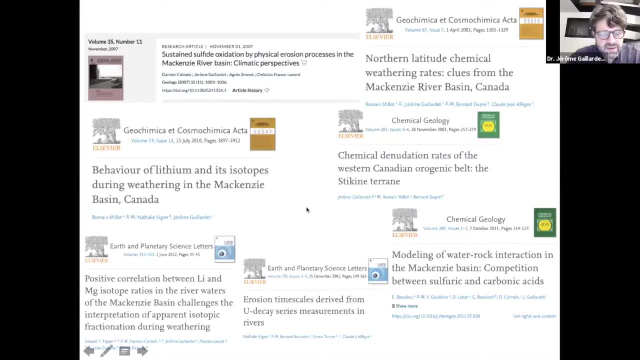 and I don't want to go into the details, but I have started working on the Mackenzie a long time ago- in 1999, maybe, 97, maybe- and a number of students of mine have prepared PhD thesis on the Mackenzie. 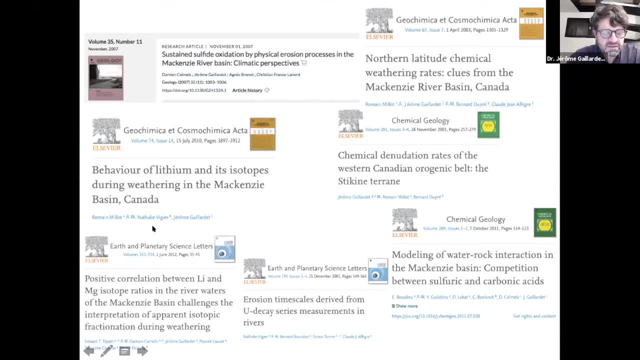 I just want to cite Romain Millot here, Nathalie Vigier and who else. Damien Kalmels did a bunch of work on the Mackenzie River also, and Mathieu Delanger most recently. So we have published a lot of papers on the Mackenzie River. 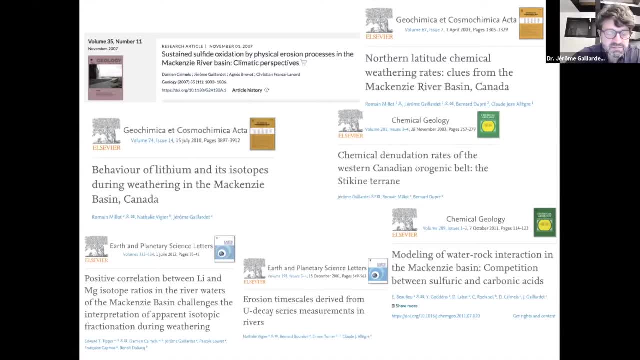 and this is why we now are able to make a complete mass budget at the scale of the catchment. So I'm going to start rapidly by saying so. I'm going to start rapidly by saying So. I'm going to start rapidly by saying: 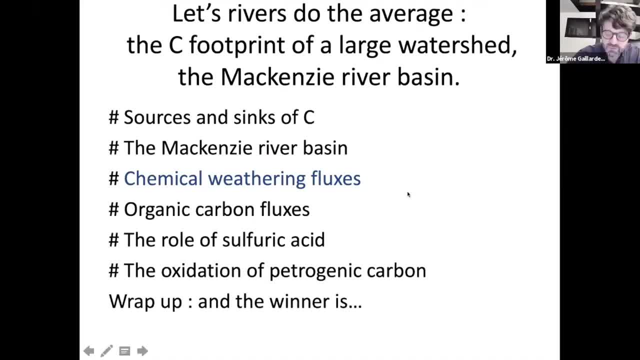 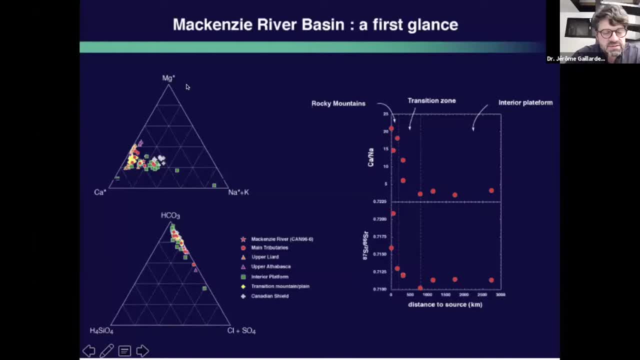 specifically by the chemical weathering fluxes. How do we determine the chemical weathering fluxes? It's pretty simple. I'm not going to go into the details here. So this is a triangle typical geochemical diagram showing you at the first glance. what is the chemical composition of the Mackenzie River? And it's very simple. basically, The Mackenzie River is rich in calcium and magnesium. It's dominated by carbonate weathering, But there is something which is very interesting, which is that the rivers from the lowlands. 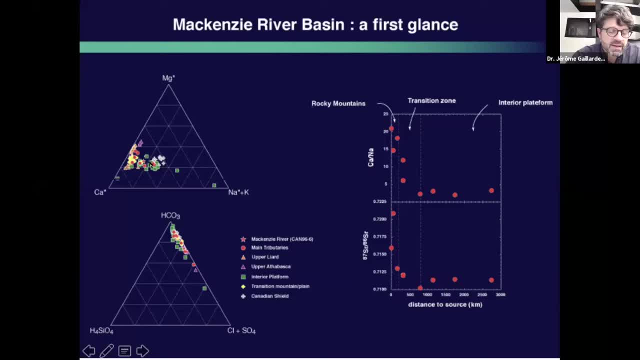 so in green on that triangle here they tend towards the silicate weathering and member which is represented by sodium and potassium on that simple diagram. This is something which is very peculiar in this catchment and which is totally the reverse of, for example. 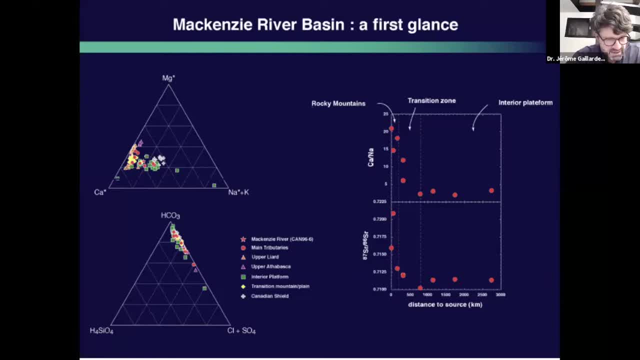 the Amazon River Basin, which is the fact that the chemical weathering of silicate is higher in the plain than it is in the mountains, And we have explanations for that, but I'm not going to go into the details tonight. And if you look at the chemical composition, 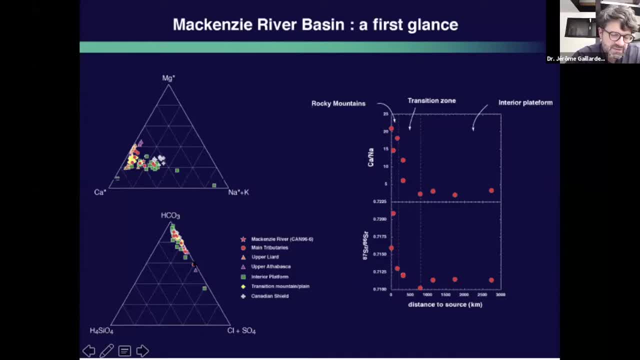 of the anions here. it's very clear also that the Mackenzie River rivers are enriched in sulfate. So the cations- calcium, magnesium, which are the dominant cations- are neutralized not only by HCO3 minus, which is bicarbonate. 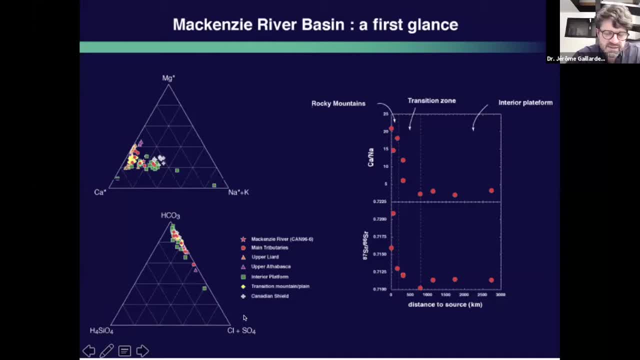 the alkalinity, but also by sulfate- And this is something important and I will come back on that later. We can calculate the amount of each cation- calcium, magnesium, sodium, potassium- which is coming from each of the dominant lithologies, based on very classical method. 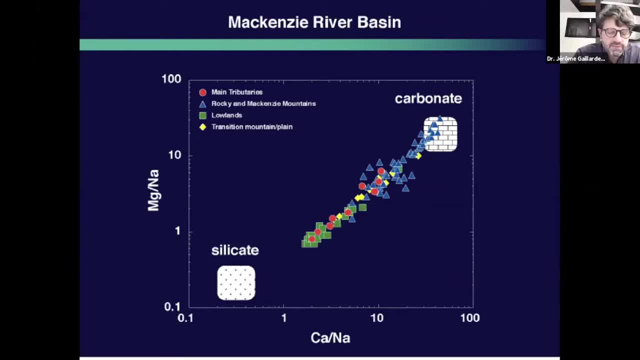 that I'm going to show very quickly here, For this is a typical mixing diagram that we use in geochemistry to calculate the contribution of silicate versus carbonate dissolution to rivers. So here you have magnesium sodium as a function of calcium-sodium diagram. 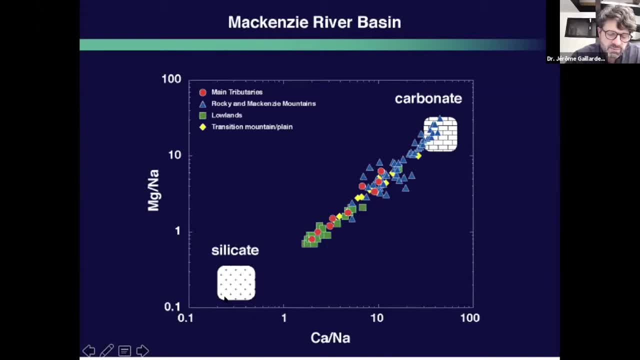 And these fields. here are the typical composition of waters draining silicates and waters draining carbonates, And you do see that the chemical composition of the Mackenzie River rivers are in between. So they are due to mixing of water draining silicates and waters draining carbonate. 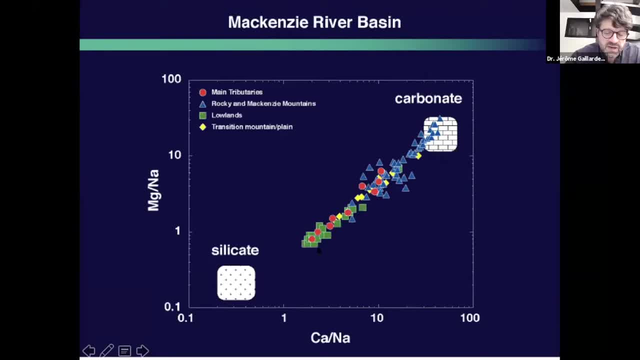 This is not the big surprise. but again, the big surprise is that the rivers from the plains, from the lowlands, are the ones which are closer to the silicate in member Meaning that these rivers which are in the lowlands, 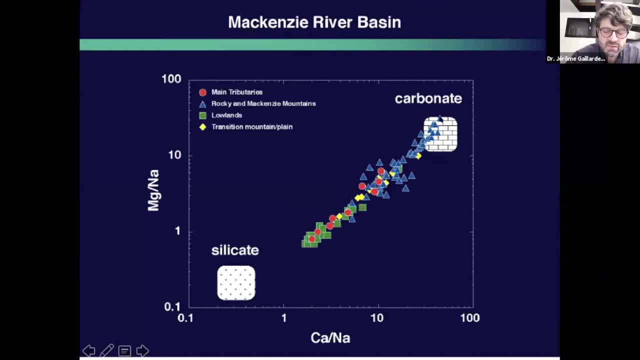 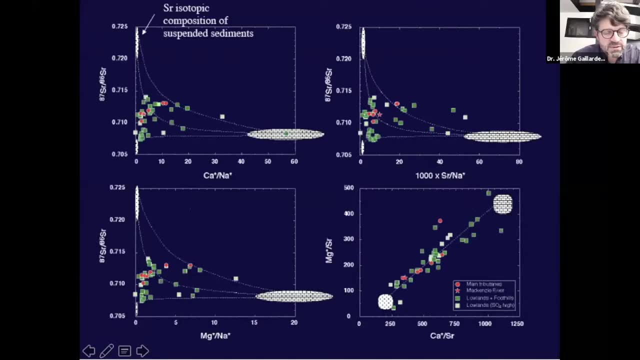 are more influenced by silicate weathering than the rivers in the mountains, which are dominated by carbonate weathering. I think I don't have time to go into the details of how we use trans-therm isotopes to constrain the origin of cations. 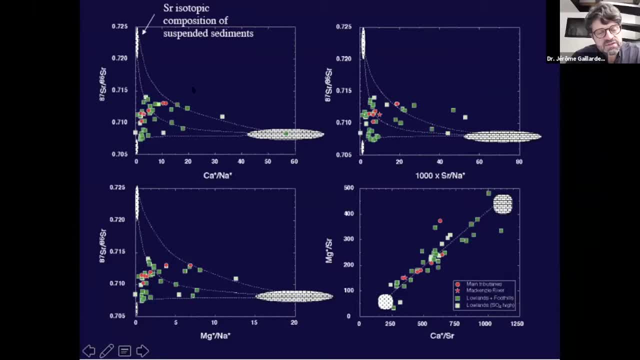 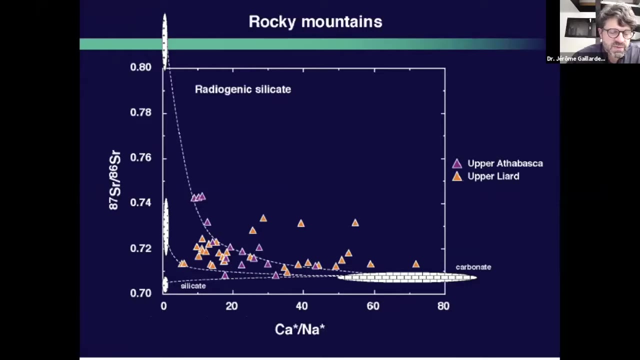 and to deduce how much of the different solutes come from the silicate in member and the carbonate in member. So I'm going to skip that. We can keep that slide for the questions. if some of you are interested, I just want to mention that in the Rocky Mountains 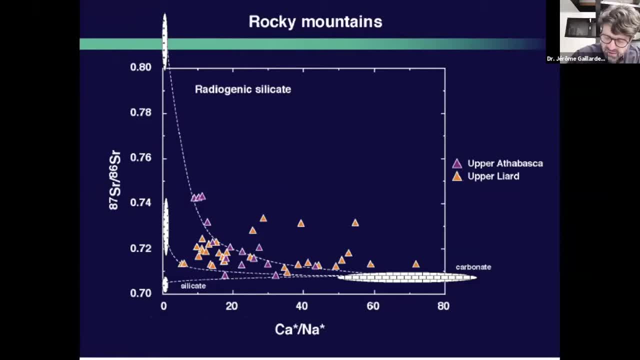 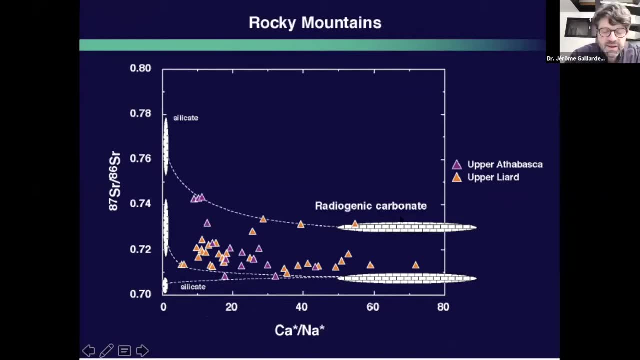 we found something very peculiar, which is that there is probably somewhere in the Rocky Mountains, but we don't know where- carbonates which are radiogenic in trans-therm, which means that these carbonates have a very unusual trans-therm isotopic ratio. 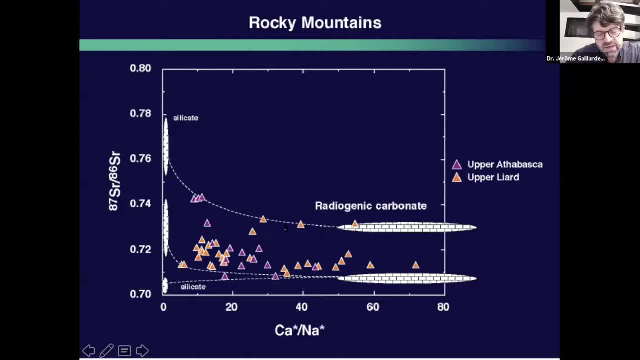 There's no way you can explain the river chemical and isotopic composition for trans-therm of these guys here, which are rivers during the Rocky Mountains, if you don't have a carbonate in member which is radiogenic. And for those of you which are familiar with the 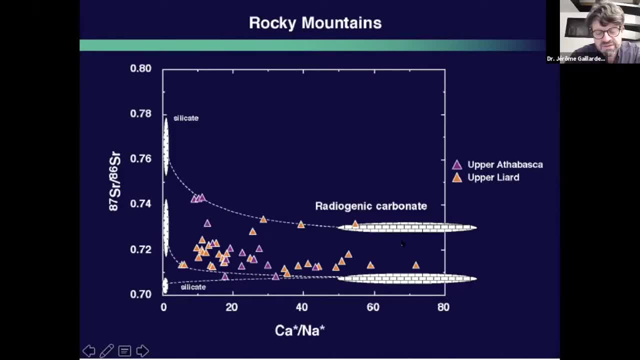 geochemistry of trans-therm in rivers. this is a case that is also found in the Himalaya. So, in a way, the carbonate of the Rocky Mountains are like the carbonates of the Himalaya: They are containing a radiogenic trans-therm component. 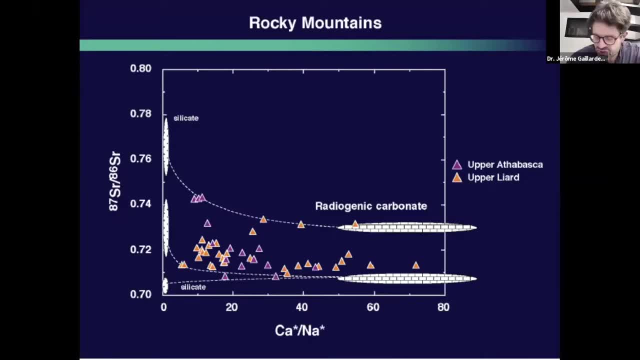 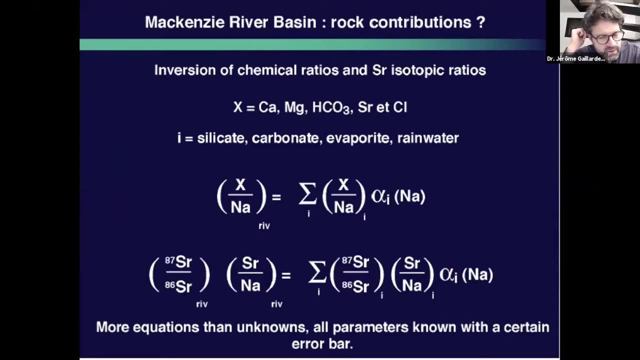 We're not sure about the origin of this radiogenic trans-therm, but for sure it exists and more work should be done on that. So we can calculate. and again I'm not going into the details here. We use an inversion procedure to basically 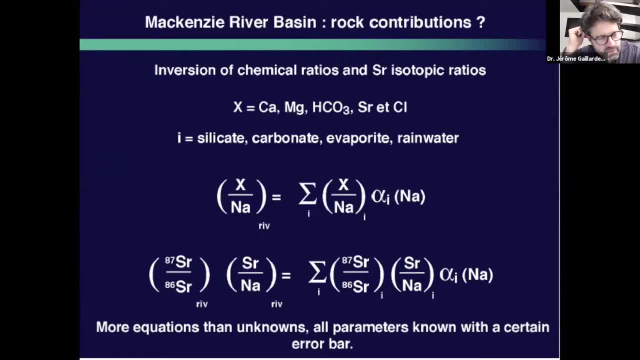 to solve the different mixing equation. So we have several tools we can use. We can use the chemical ratios, We can use the isotopic trans-therm ratios, And so we have a lot of information on the way the mixing between the different lithologies are made. 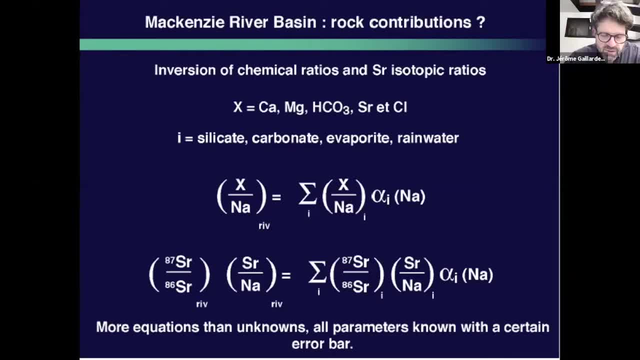 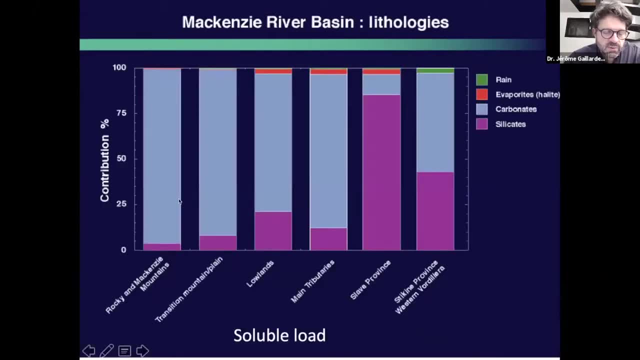 And this system, which is an underestimated system, can be solved using an inversion procedure And at the end we are able to calculate for each of the big regions here: Rocky Mountains, lowlands, the fall lands, basins, the main tributaries of the slave province. 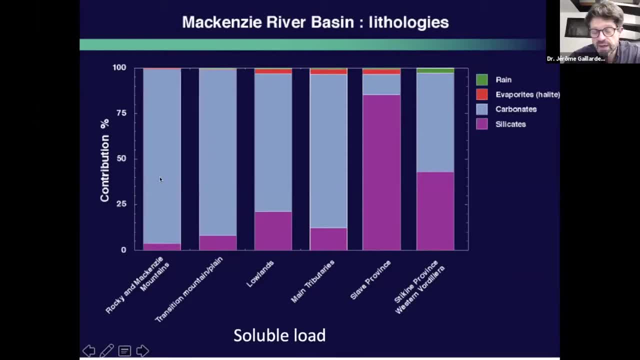 we are able to calculate how much of calcium, magnesium, sodium and potassium is coming from each of the lithologies that we have evidence on the mixing diagrams. Okay, so basically the model here is assuming a mixing between rain which is not contributing too much. 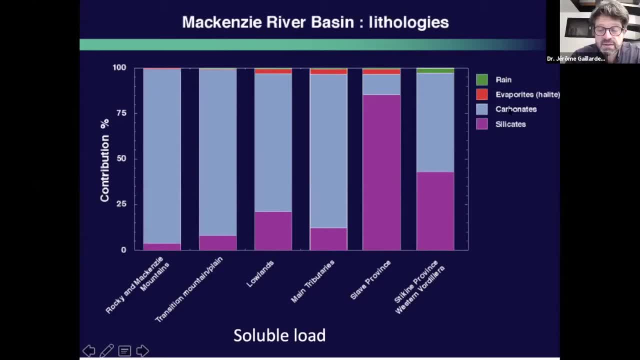 evaporites evaporitic rocks that exist within the Mackenzie River Basin, carbonate and silicate rocks, And so we are able to save that, for example, in the Rocky and Mackenzie Mountains, and then most of the soluble load is derived from carbonate weathering. 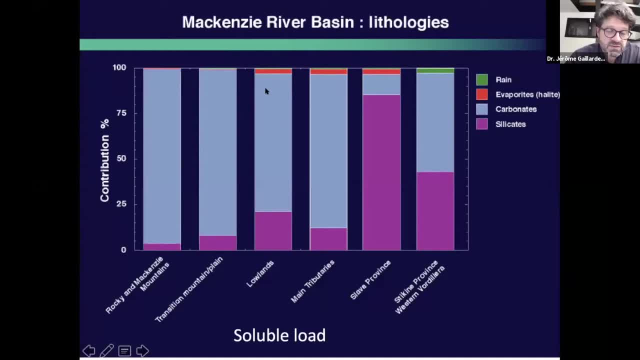 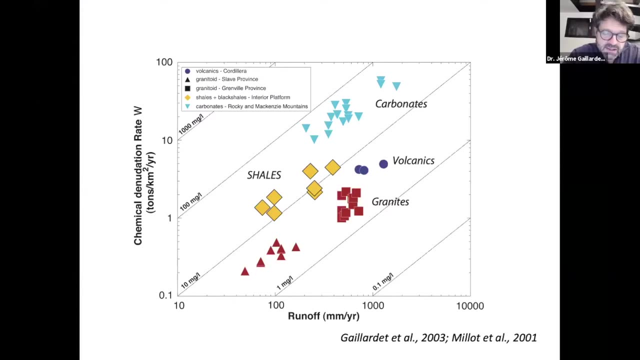 But in the lowlands this contribution of carbonate weathering is less and the contribution from silicate weathering is higher. So why is it important all this calculation? It is important because I want to calculate the amount of CO2, of atmospheric CO2, which is consumed. 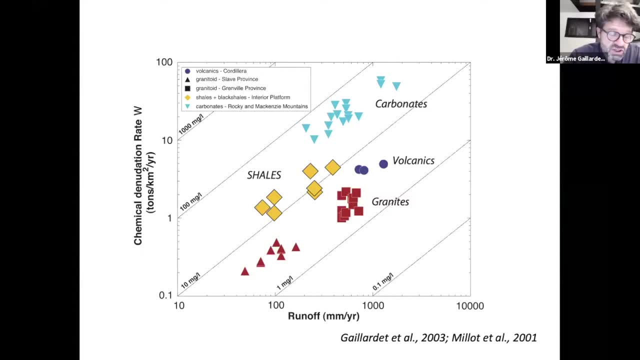 by the reactions: the weathering reactions involving carbonate or silicate, because, as I showed you before, if you weather silicate or if you weather carbonate, the consequence on the global carbon cycle are not the same, So you must be able to distinguish. 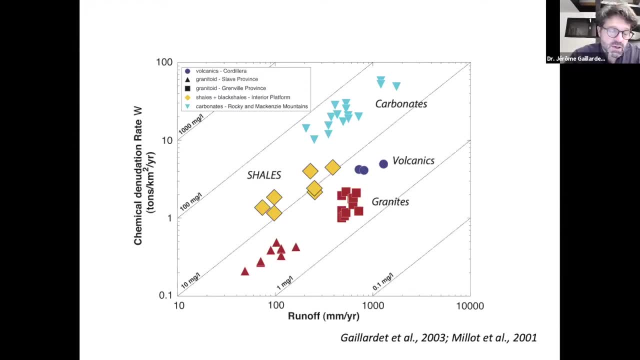 between the two lithologies And this is what I have summarized on this diagram. So it's giving the chemical denudation rates, or I could have showed you the CO2 conception rate. It's the same. It's proportional as a function of runoff. 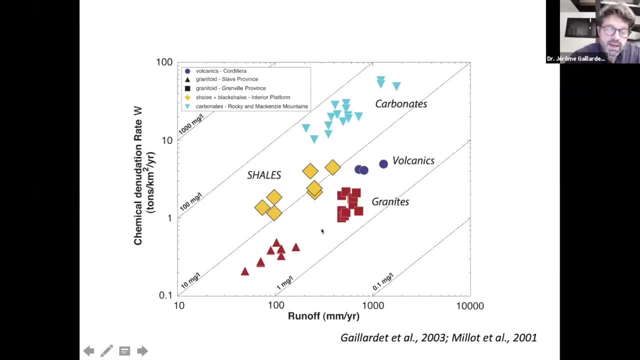 Runoff is basically the river discharge And you do see that there are big difference between the different regions and this corresponds to different lithologies. It's not a big surprise that carbonates have higher denudation rates than the granites of the Shell province. 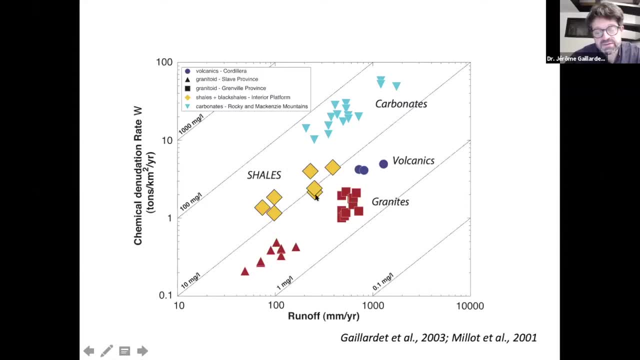 But what is interesting here is to say that is to show that the shells which are in the lowlands have weathering rates and then CO2 conception rates which are higher than the granitic rocks. This is not something which is general at the global scale. 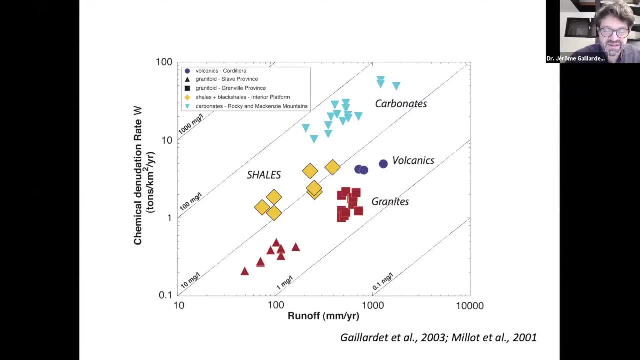 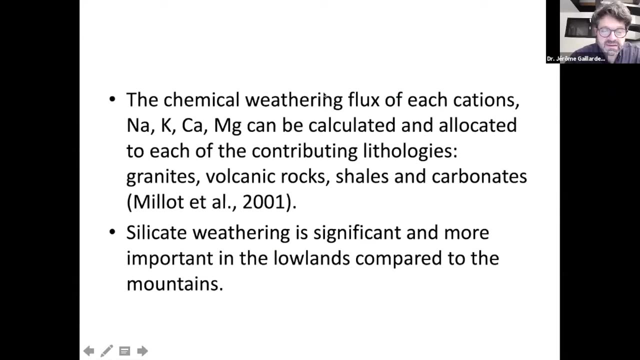 It's, in a way it's a peculiarity of the Mackenzie River basin. Okay, so, to summarize, we can calculate based on the inversion of chemical data. We can calculate the chemical weathering flux of each cations: sodium, potassium, calcium, magnesium. 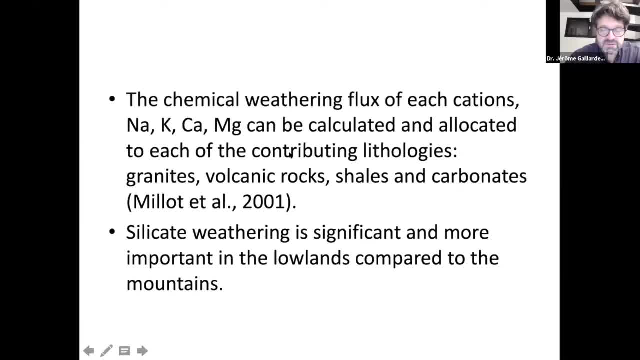 and allocate the different ions to the different contributing lithologies. This has been published by Miguel et al in 2001.. And so silicate weathering is significant, So it means that there is some CO2 which is consumed, even if the temperature is low in that region. 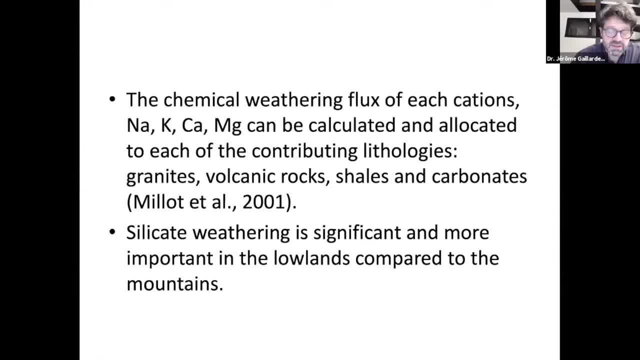 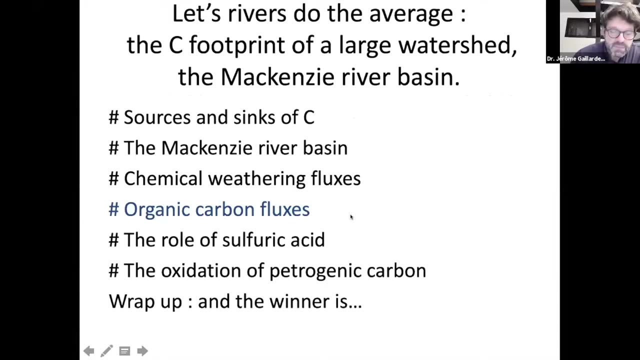 in that part of the world Silicate weathering is significant, And that's probably due to the long residence time of water in the swampy areas of the lowlands. So let me now turn to the organic carbon fluxes. So how do, how can I do that? 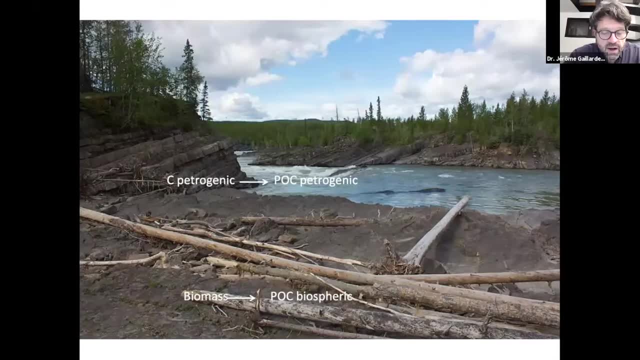 So in a river, you have two types of carbon: organic carbon, which is transported. You have carbon which is basically modern Meaning, that is, carbon from the present, current ecosystems, which has been physically removed from from the landscape and is going to reach the ocean, transported by the rivers. okay, and this is 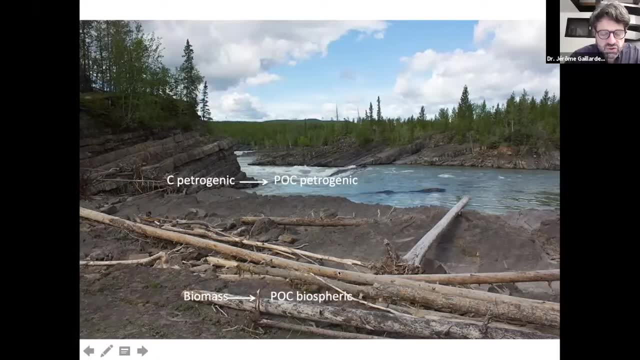 typically the case for these trunks that i'm showing here. but you have another source of carbon, which is what we call the petrogenic carbon, which is actually fossil carbon, which is contained, for example, here in these sedimentary rocks which are outcropping on the bank of the river and when 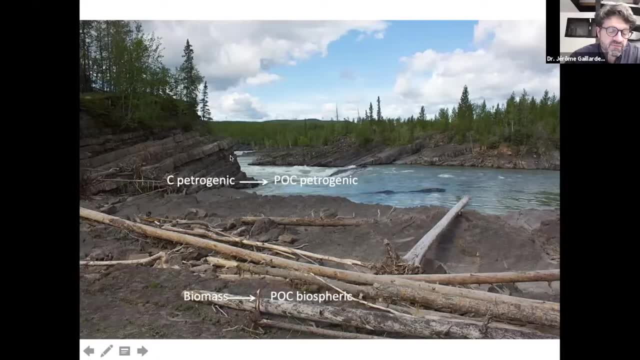 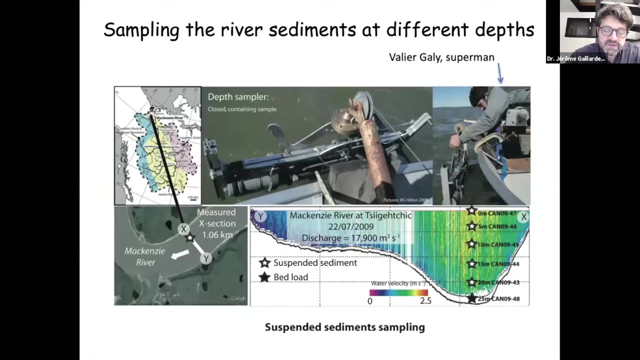 the river is eroding the banks, then some some fossil old carbon is going to be transported, and so if i want to make a proper carbon burial budget, i need to distinguish between the two. and this is what, in mackenzie, we're using. i'm not going into the details, but we are using deaf. 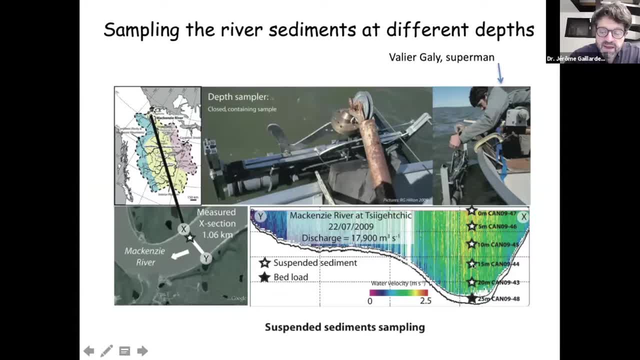 profiles where we sample with depth the different suspended sediments and by doing that we get access to a range of size. we have a gradient, a gradient of a grain size that allow us to work on several types of sediments. the bottom sediments are usually coarser. 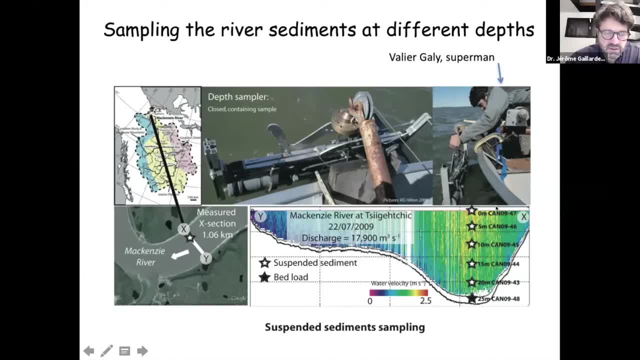 than the sediments which are transported at the top of the river. here is my colleague, bali gali, that some of you probably know, which is a real superman. if you need someone to carry very heavy material on a boat and do impossible things, he is your man, and so we did. 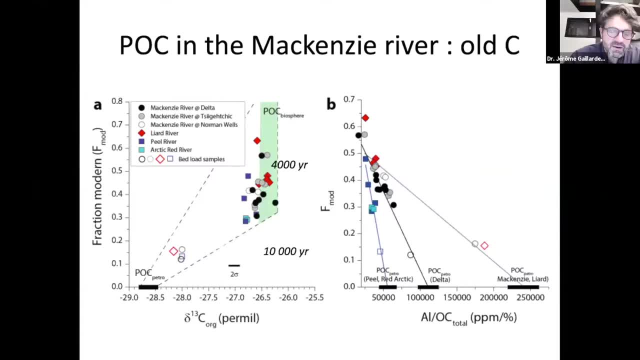 with bob hilton we did carbon 14 to identify, to distinguish between these two source of carbon. why? because the modern carbon contains, contains carbon, which is carbon with a significant amount of carbon 14, but the petrogenic carbon doesn't, does not contain any carbon 14. because this carbon is dead, because 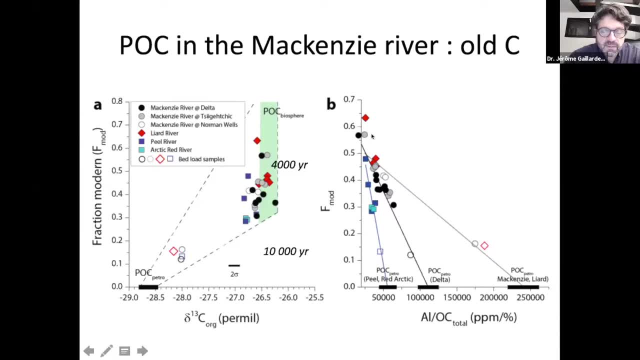 this is old organic matter and so not going into the details here, but basically using the depth profile we are able to see that for the different tributaries of the mackenzie river- here at the peel, the red arctic, here is a mackenzie and the lyard river- we can calculate how much of the 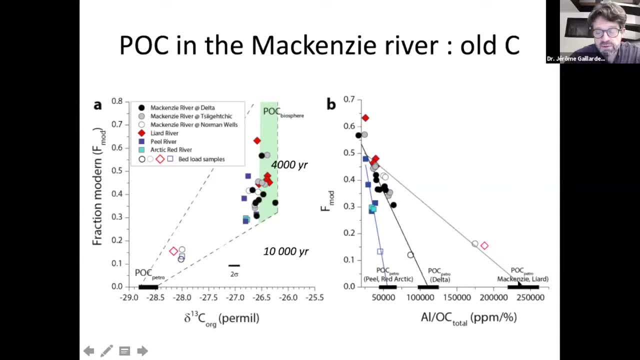 organic carbon is petrogenic, so old carbon. and how much of the carbon in the sediments- i'm talking about this, the sedimentary load here to particulate load? how much of this carbon transported into the solid phase is modern, okay, and and so we we see here in the mackenzie. 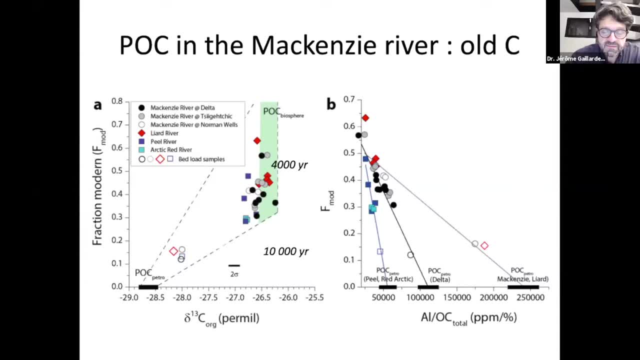 and it was very interesting to see. that is that the you have. you have a mixing for each of the tributaries, uh, visible on the depth profiles. you have a mixing between um, old carbon, so fossil carbon, which is preferentially transported at the bottom of the river, and modern. 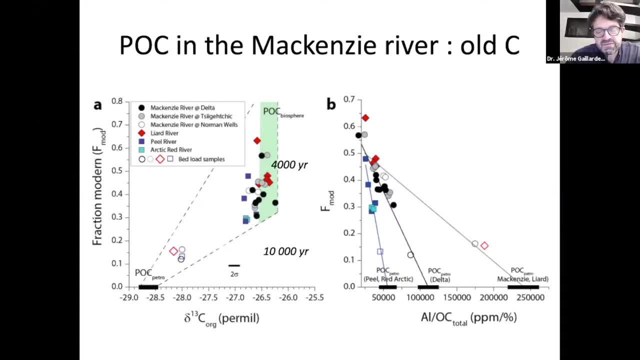 carbon, which is not really modern, because if it would be modern it would have been a fraction of one, but you do see that it's not one, it's 0.4.5, meaning that this carbon has an age. actually, and if you calculate the age, that's that this carbon transported at the surface of the river in the. 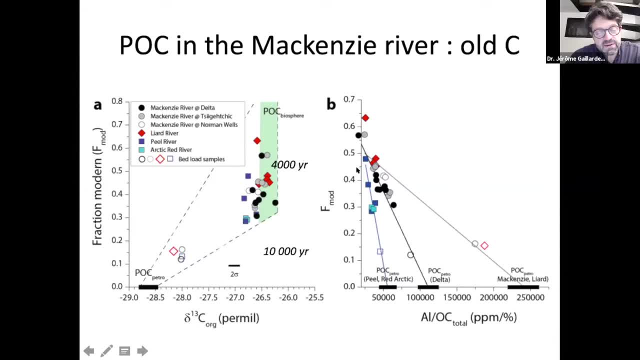 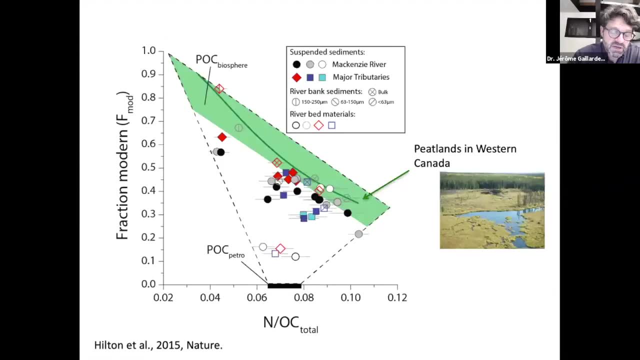 sediments uh should have. it is something like uh, five, four or five thousand years. so this is one of the findings, uh of the paper that was published with with hilton in nature a couple of years ago: that the mackenzie river is transporting biospheric carbon to the ocean. 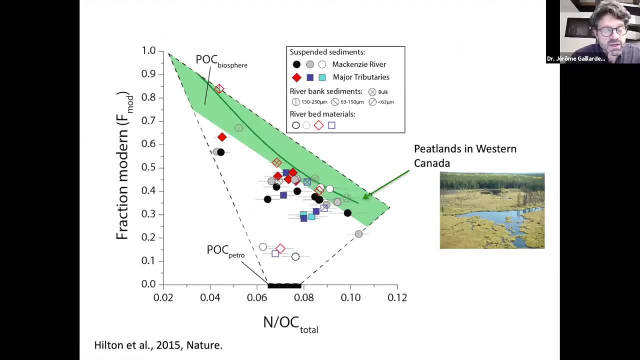 but this biospheric carbon is is not new. it's carbon which is derived from the peatlands- uh, peatland areas of the catchment, probably, or the size of the catchment- and which is basically old- okay, we are releasing carbon dating back from 5 000 years and now this carbon is being transported to the ocean and, of course, 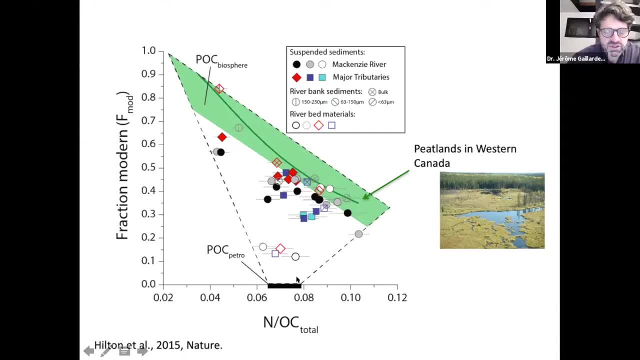 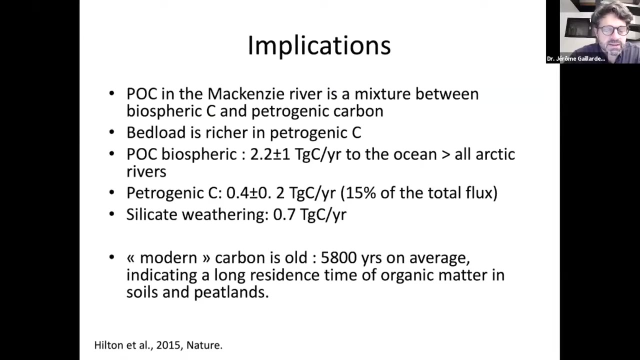 we are also transporting old carbon, petrogenic carbon, that we need to correct to come up with a flux of carbon- burial carbon, organic carbon sequestration- and so this is a calculation that we did and so we are able to calculate a flux. i'm not going into the details here of the numbers. 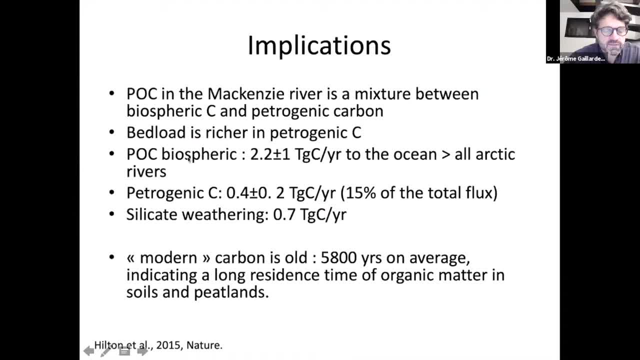 a flux in teragram of carbon per year of biospheric carbon, which is transported to the ocean, and petrogenic carbon, which is transported to the ocean. but just let me uh notice that 2.2 teragram of carbon per year are represented by particulate organic carbon of biospheric origin. 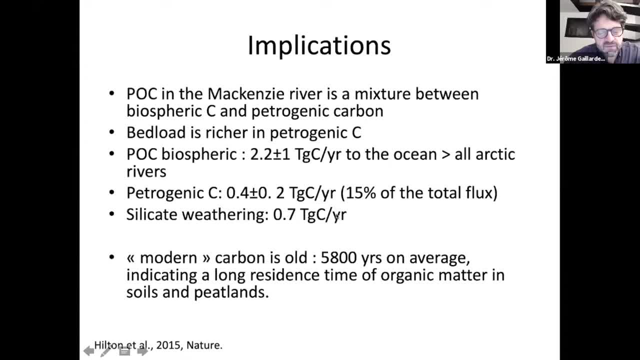 and so you can see that the silicon silicate weathering is consuming 0.7 teragram of carbon per year- the numbers that i've showed you before- and and so you do see here very clearly that the sequestration of organic carbon is much more efficient. 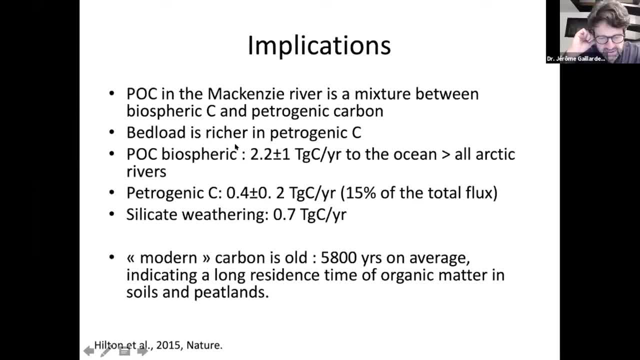 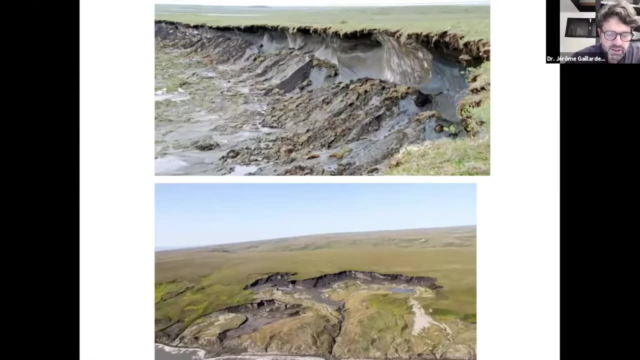 than the sequestration of inorganic carbon by silicate weathering, and this carbon is not really modern, it's old but i'm not going to uh detail that tonight. So probably landslides, which are occurring everywhere in the Mackenzie Basin and which are more important now because of global warming, are probably releasing carbon which was sequestered in the soils, in the peatlands and putting this old carbon, or modern but not really modern carbon, into the river. 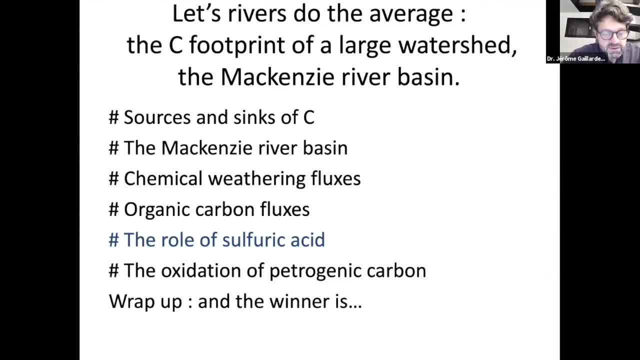 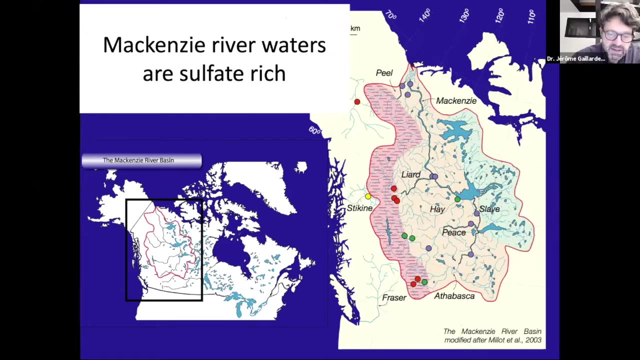 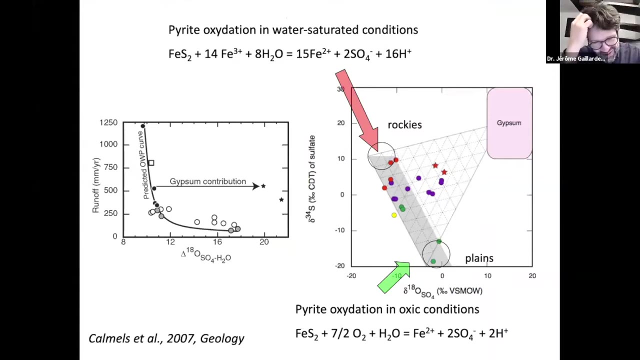 Okay, so an important process in the Mackenzie is due to sulfuric acid And, as I showed you before, the Mackenzie River waters are rich in sulfate And, with Damien Calmel a couple of in 2007,- it's not a couple of years anymore- ago, we published a geology paper in which we showed that this the origin of the sulfur. 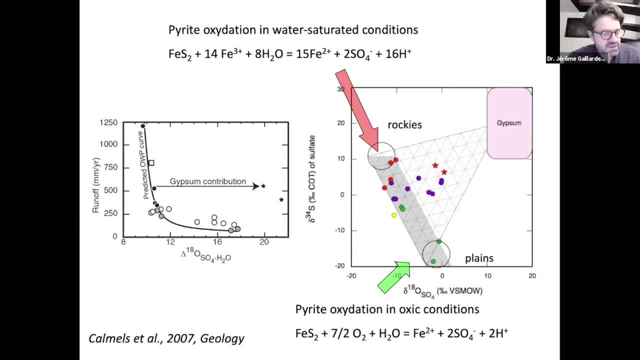 was sulfide oxidation. I'm not going to go into the details here. You can read the paper if you're interested. but basically the idea is that we can use sulfur isotope and the oxygen isotope of the sulfate molecule to constrain the origin of the sulfur, of the sulfate which is dissolved in the river. 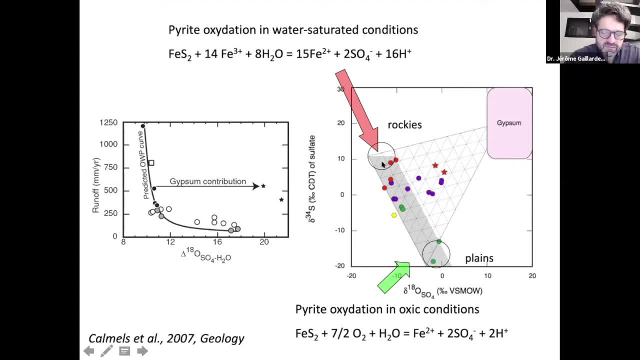 And you need. you need the two isotopic ratio. If you just want to get one information- sulfuric acid, sulfur isotope or the oxygen isotopes- you cannot be conclusive, So you need the two. And this diagram here, which is a plot of sulfur isotope as a function of oxygen isotopes from the sulfate molecule, shows clearly that most of the sulfate is derived from the oxidation of pyrite in two, in two conditions: anoxic or anoxic conditions. I'm not going into the details. 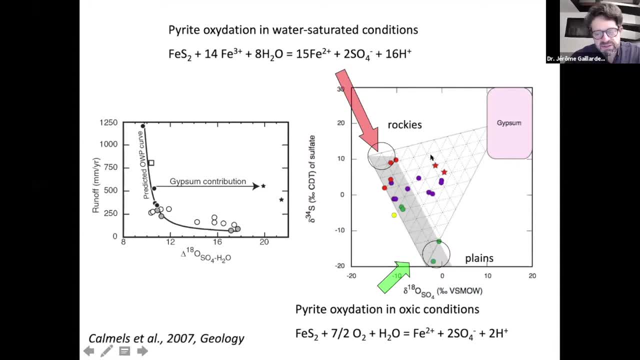 But that for a couple of tributaries, in particular tributaries in the in the Rockies, you need some sulfate coming from gypsum And, of course, if I want to, to determine the amount of sulfuric acid which has been used by chemical weathering. I need to get rid of this sulfate coming from gypsum because I don't want to include it into the weathering budget. 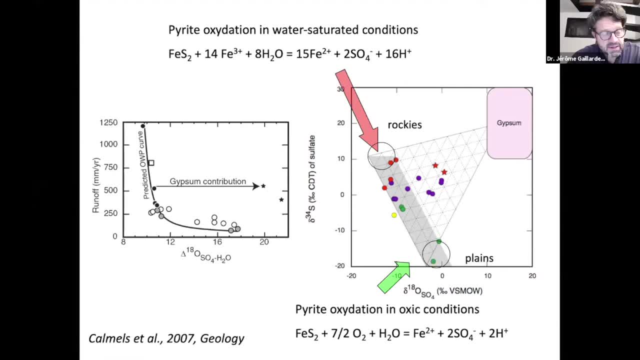 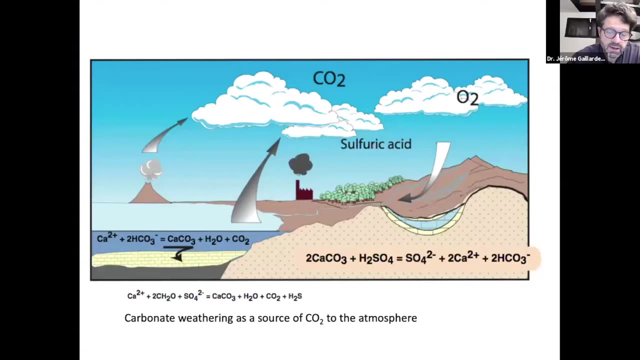 Okay, This, this is sedimentary sulfate and it's not derived from the oxidation of pyrite in the in the critical zone and it's not contributing to carbonic weathering. And this is what we did in this paper And we were- we were able to show that in the Mackenzie River. 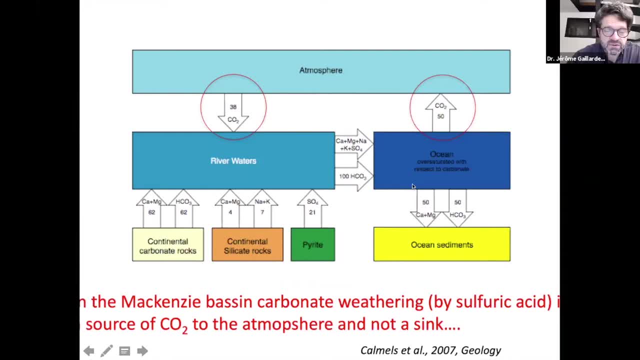 for if you, if you have, this is relative units. Okay, so this is basically the atmosphere, the river, This is the water, the ocean. So we calculated that if you, if you get 100 moles of HCO3 minus reaching the ocean from the Mackenzie River, then 38 have been consumed from the atmosphere, but because the main mechanism is not weathering of carbonate by carbonic acid. 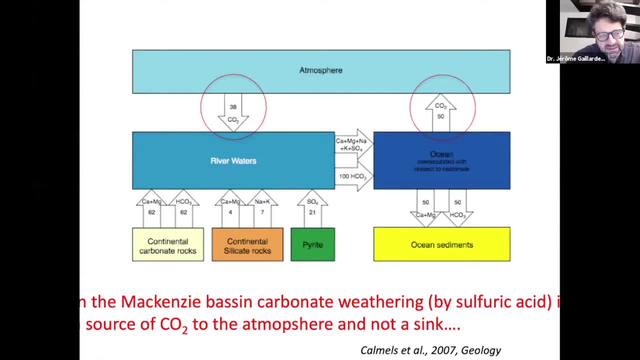 Okay, By the weathering of carbonate by sulfuric acid, it's producing CO2, according to the reaction that I've showed you before, and that's producing CO2 to the atmosphere and the number is 50.. So you do see that you have consumed, by by carbonate weathering using carbonic acid, 80, sorry, 38 percent of the CO2, but you are removing 50 percent. 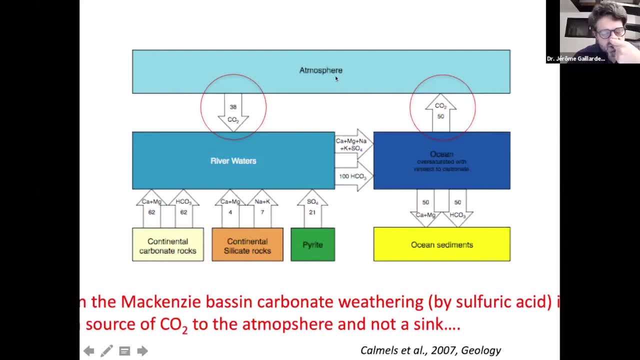 Okay, So on the on on the net budget, the weathering of carbonate is a source of CO2 in the catchment. This is what we published in in 2007 in the geology paper, which was one of the first mass budgets done on carbonate weathering, by distinguishing between sulfuric acid and carbonic acid. 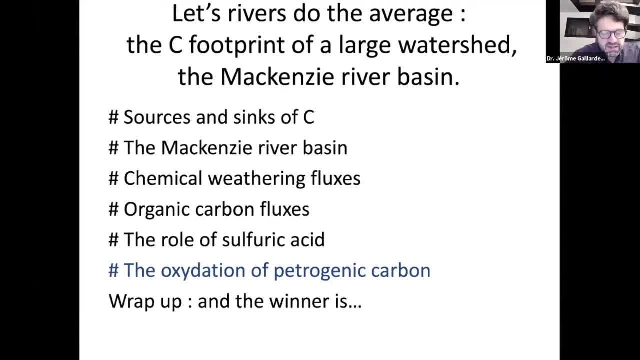 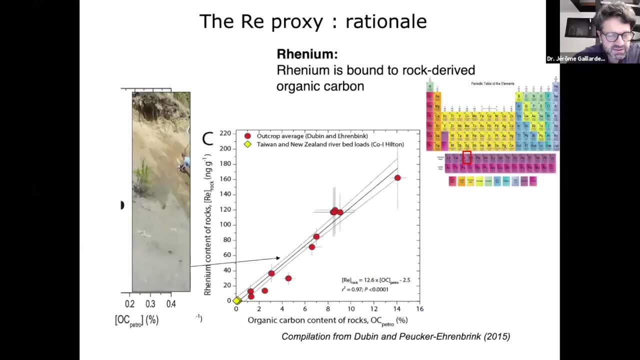 And then the last term of the of the mass budget is the oxidation of the petrogenic carbon. How much of carbon is being oxidized by the oxygen, the oxygen of the air, and is producing CO2? This is really a difficult flex to to calculate, to constrain. 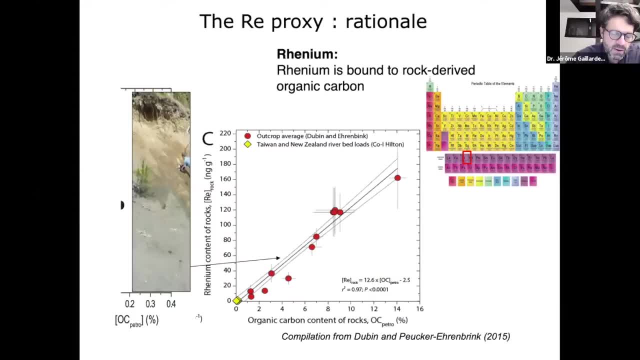 And here I'm going to show you a work that has been done by, by Mathieu Deslinger, in Durham and Paris. This is very interesting. Okay, paris, which is to use rhenium. rhenium is a very rare element, it's difficult to measure, it's very. 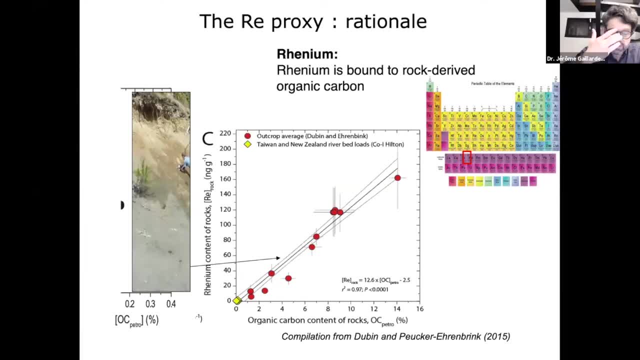 low concentrated. it's a platinoid, but it has a very interesting property, which is that it is coming with organic matter in a rock. so here you have a compilation which was published by by the woodsell group a couple of years ago, which show that in a sedimentary, in sedimentary rocks, 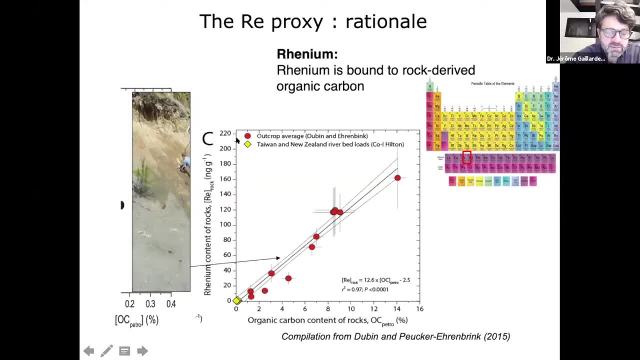 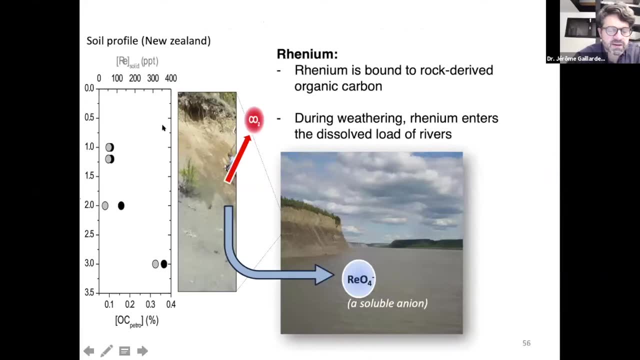 the more carbon, organic carbon, you have, the more rhenium you have, the concentration increases with a common content. and when you look at the soil profile- and this is a soil profile developed on a organic rich bedrock- here you do see that the rhenium is decreasing very much. when you 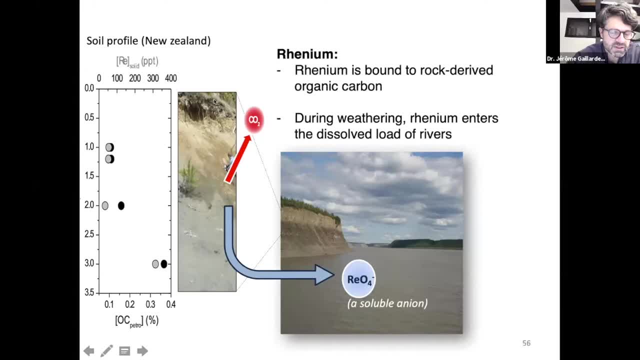 enter into the weathered zone here, where the organic matter has been oxidized, and this is not a big surprise, because rhenium is a very soluble element and which is transported in rivers as an anion. it's very low concentrated, but it's very soluble, so we maybe we have the good tracer. 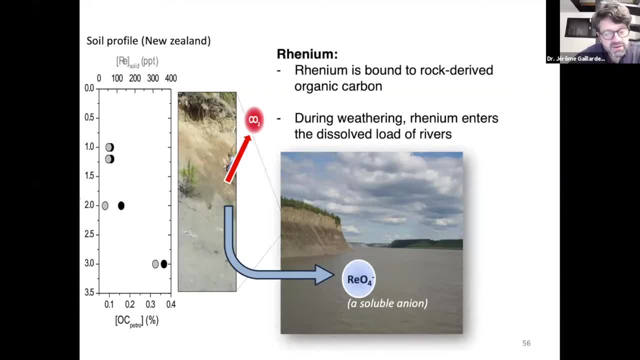 that will allow us to quantify the oxidation of organic matter in the landscape. because if we are able to measure rhenium in the mackenzie or, in general, in rivers dissolved in river, in rivers, then you can, we can get an idea of how much organic matter has been oxidized at the scale. 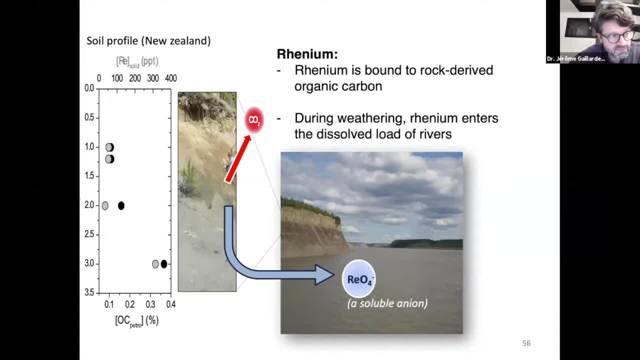 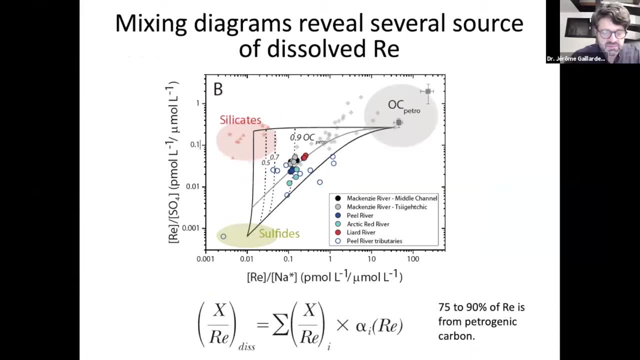 of the watershed and we can. we can come up with a flux. this is basically the idea. it's a bit more complicated because in geochemistry it's always a little bit more complicated, but we have methods a little bit more complicated to measure rhenium and this is a very interesting study and it's 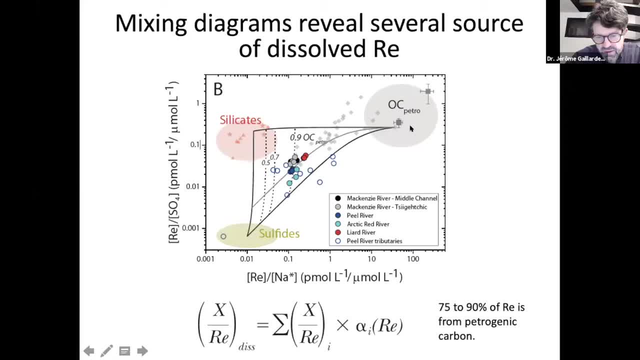 actually a very good research and effective study of organic matter, and we're doing a lot of research for organic matter, and the thing that we're doing is we're doing a lot of research on how to measure rhenium and i'm going to show you the data that i have here. but what is i'm doing is i'm using 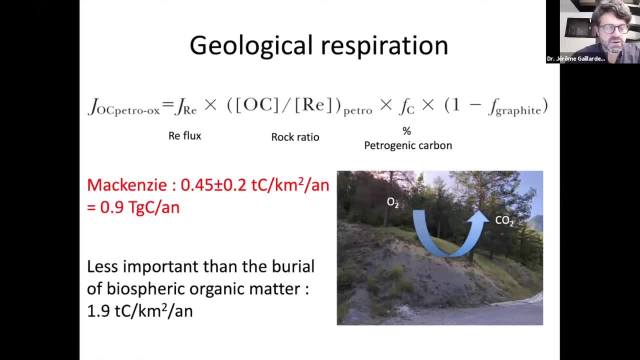 the rhenium and the solid acid and the sulfide, and the rhenium and the sulfide, because this is not always the case. but this is a way of doing this and the method that we are doing us to distinguish CO2 produced by the respiration, which we call the respiration of things. in other words, in other 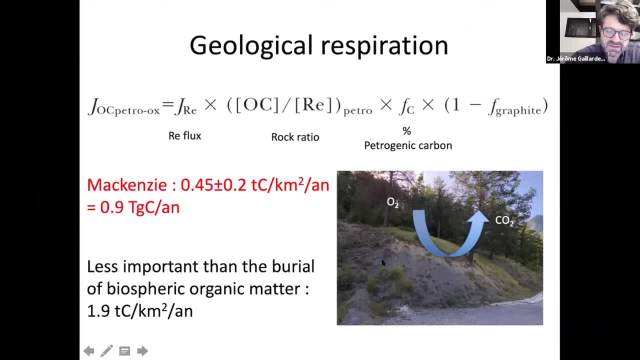 words, the transformation of organic matter from the bed, from the sedimentary rocks, uh, into CO2 and and and. so this is uh you can, you can see in the paper, you, you will find in the paper the details. but the flux that we calculated for the Mackenzie river at mouth showed that there is a 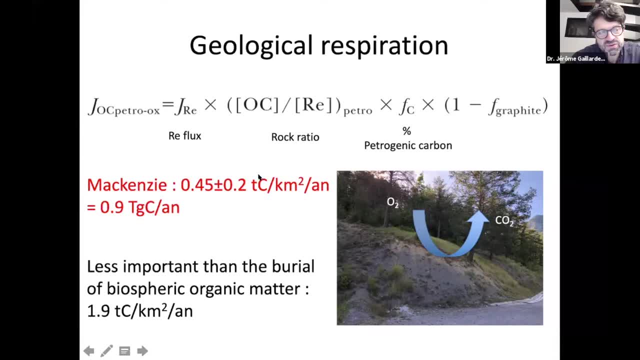 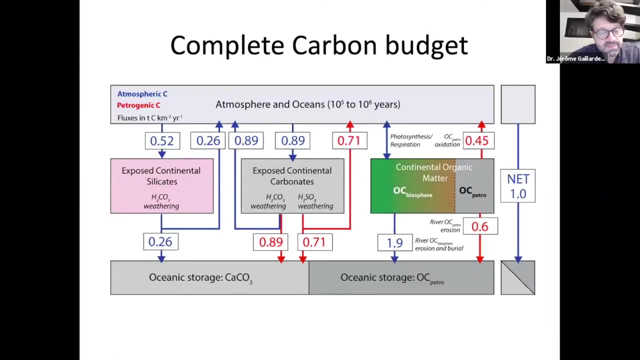 significant amount of CO2 which is produced this way. it's still lower than the carbon burial, but it's not. it's not negligible. so I now come to my almost final, final slide, which is: which is which, which is the which is the winner is: is the Mackenzie river source of a sink of CO2? and this is summarized on: 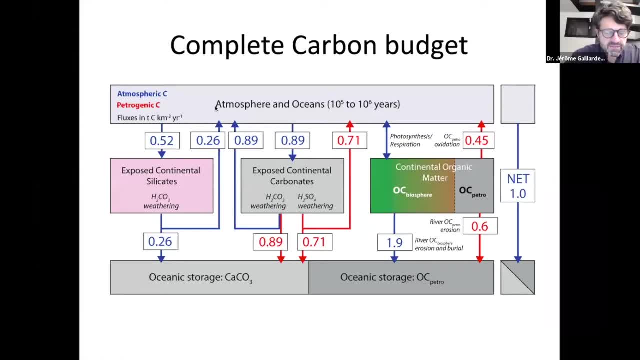 this slide when I have, where I have put all the inputs and outputs to the atmosphere, an ocean system by the different mechanisms that I have explained to you earlier. okay, so just an example. this is the amount of CO2, point nine, point nine, eight, nine, oops, eight, nine here- which is consumed by carbonate. 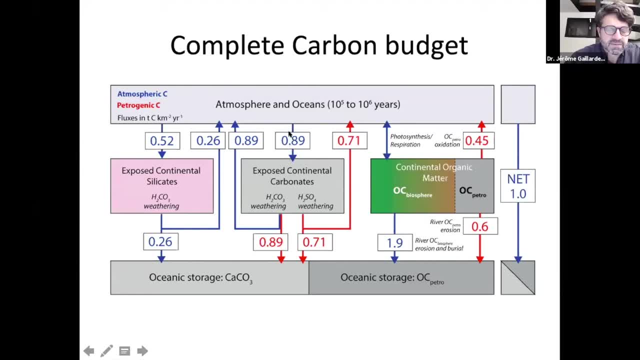 weathering. but, um, this is the CO2 which is consumed by carbonate weathering, but this is compensated by a equal amount of CO2 which is returning to the atmosphere, just because this is carbonate weathering. this is a silicate. uh, sink, uh, this is the carbon. 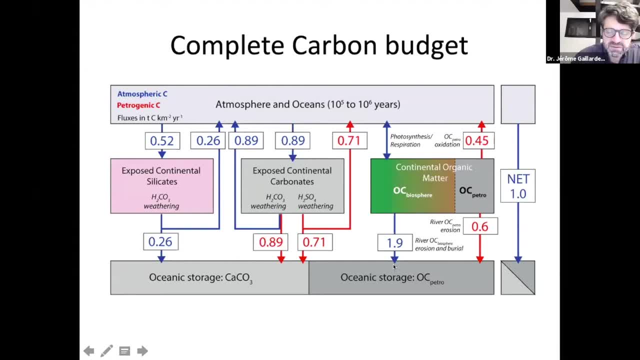 nodalating. so this is the carbon nodalating, and that's why this is so important: that you, you can keep track of the amount of CO2 in the atmosphere and the flow rate, and the amount of carbon in the atmosphere is still very low, um, and so what we would then be able to do is we're 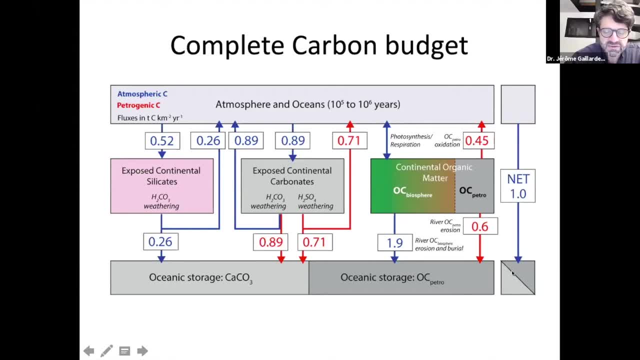 going to look at the energy activity rate and the the energy distribution rate of the ocean, and if you look in the upper right part of the slide, you can also see that the other side of the graph- that is what we just look at, is the energy rate of the ocean, and we'll go back and see what's. 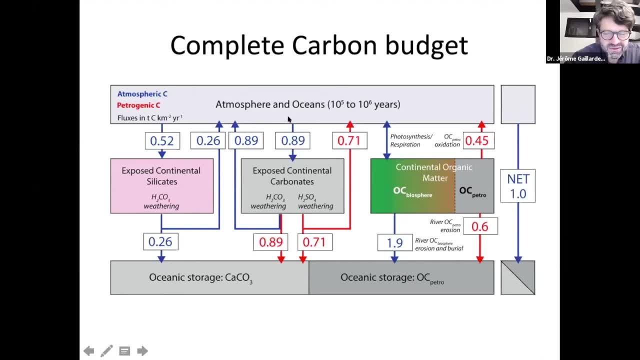 is the energy rate of the ocean and we'll go back and see what's the current energy rate of the ocean valid. the Mackenzie River catchment is still is a sink of CO2 from the atmosphere. okay on a long-term perspective. 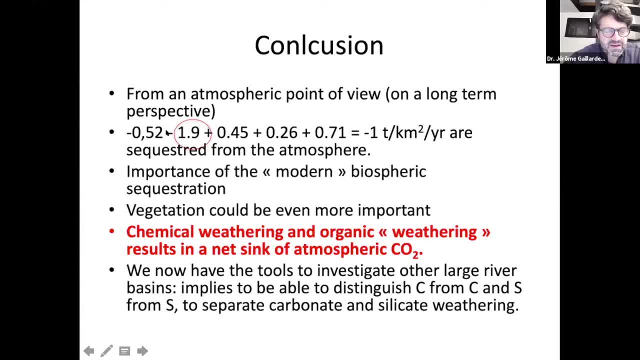 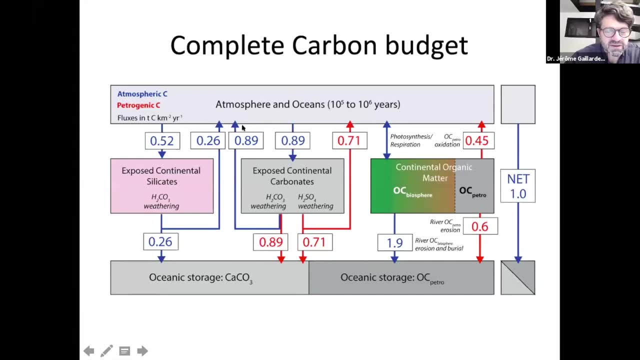 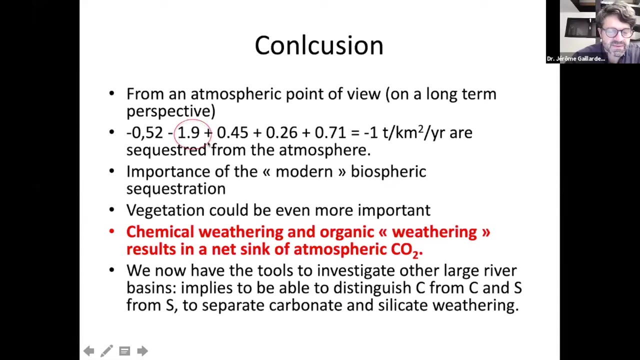 And so this is the detail of the calculation, And you see that this equation that allows you to calculate the minus one, which is the one ton of carbon per square kilometer per year, this calculation strongly depends on this term here, which is the highest term of the equation. 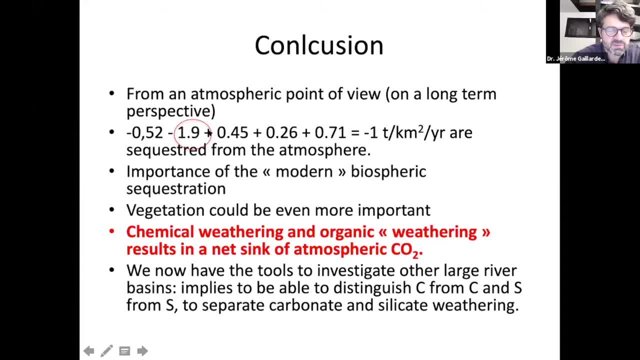 And this term is what This term is: the organic burial. okay, So this calculation shows that the modern biospheric sequestration is the most important term of the budget And if you change it, then you're going to change the net conception or emission of CO2 from the catchment. okay, 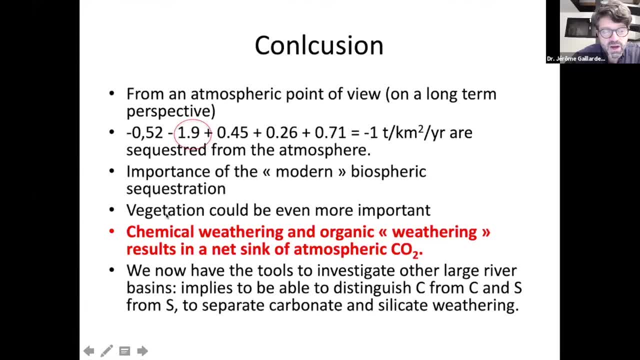 So if you have more vegetation, for example, if you warm up the climate, vegetation will grow up and probably organic carbon burial will increase And then you will increase this flux here And so maybe you will change the global, The global mass budget of the McKinsey in terms of CO2 conception or emission. 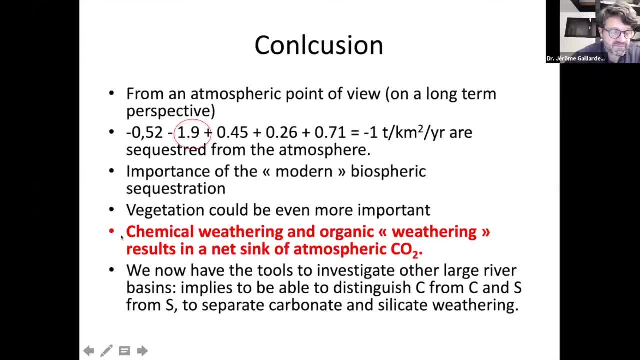 Okay, So the conclusion of the study is that chemical weathering and organic weathering are results. both results in a net sink of atmosphere. We have, as I showed you, tools to investigate, for all the large river basin, this kind of approach. 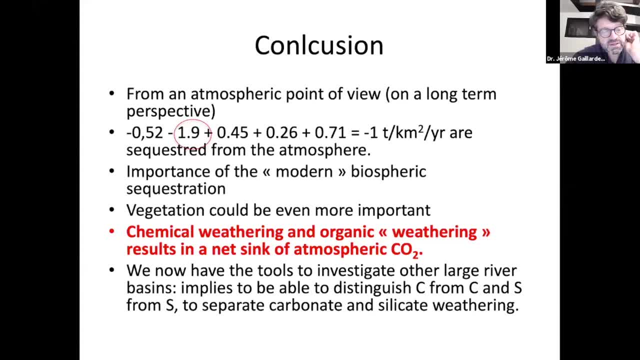 And this is what. This is what is needed now, because we don't have a global idea. okay, We don't know what at the global scale, When we will combine all these processes: CO2 conception by silicate, weathering, the. 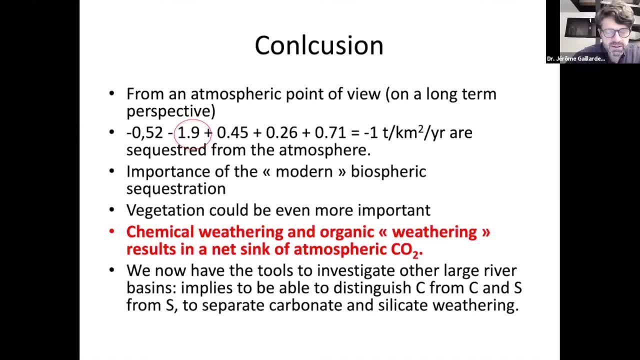 use of sulfuric acid to weather carbonates, organic burial, petrogenic carbon oxidation. we don't know at the global scale what will be the result. Okay, Thank you, Thanks, Thank you, And many of our colleagues are still working on that issue. 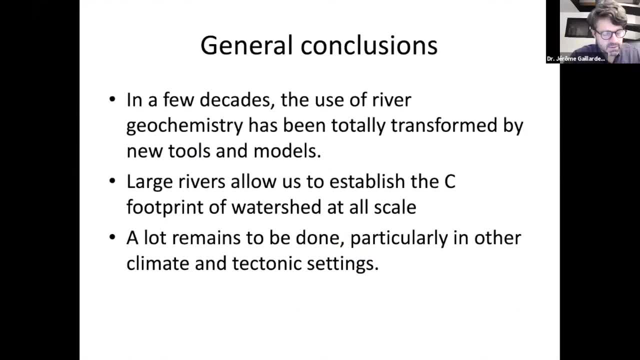 Some people, for example, Mark, is working on that problem in the upper Madrid Idios airport tributaries, on the Amazon Of the Amazon, And so we. The conclusion I'd like to give here is that we have the tools okay. 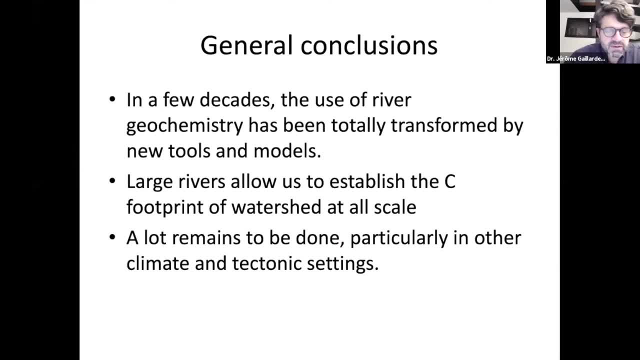 We The rhenium is probably not perfect, It's not the best solution- Okay, a perfect tool to deduce the amount of carbon which is being oxidized, petrogenic carbon which is being oxidized- but it's not bad and it's working, I think, quite well. 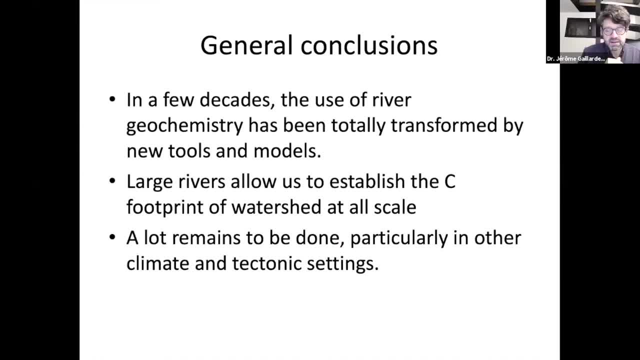 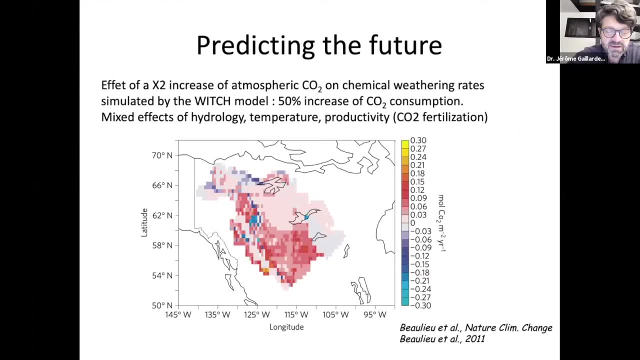 And so we need to do that at a larger scale. There is one paper which was published last year actually was published exactly at the same time as we published our paper on the Mackenzie. This is a paper by. I don't have the reference here. 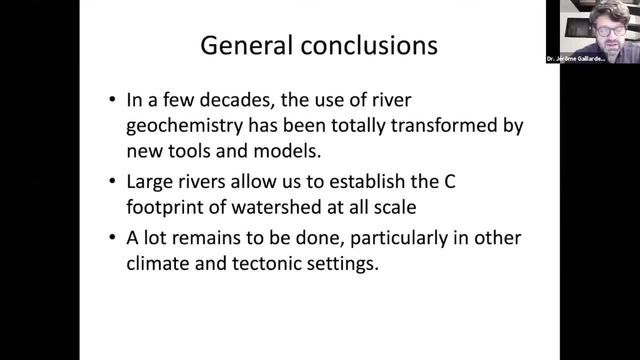 It's a paper by the group at ETH. We calculated the same kind of carbon budget that I've showed you here on a smaller watershed in Taiwan, And the result is exactly the one that I have showed you here: A big importance of organic carbon burial. 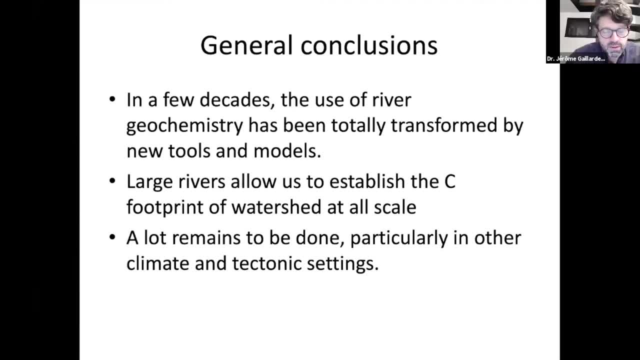 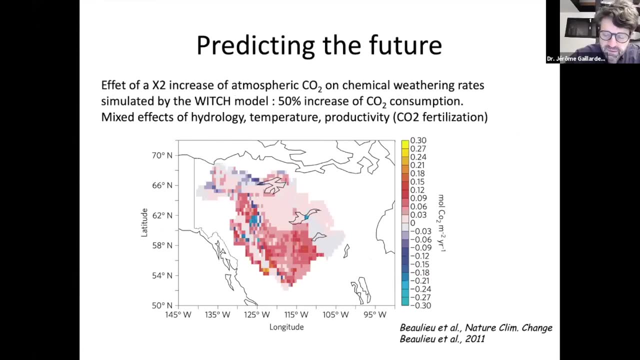 but on the whole, on the whole, the catchment is still a sink of CO2, a sink of atmospheric CO2.. So I think I'm going to stop here, just by this slide. In 2011,, Yves Goderie's team published this paper: 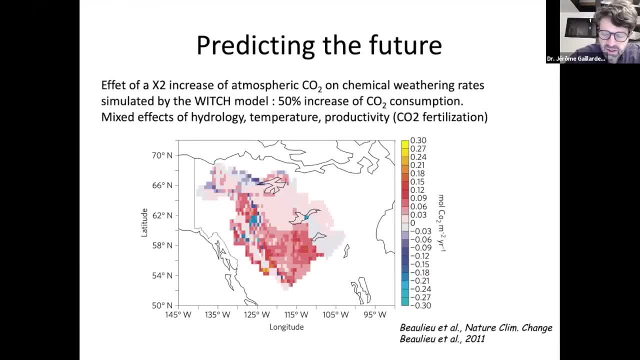 in Nature Climate Change. It's, according to me, the first. according to my knowledge is the first paper that a river geochemist have ever published In nature climate change. okay, Meaning that climatologists are starting to realize that rivers are important. 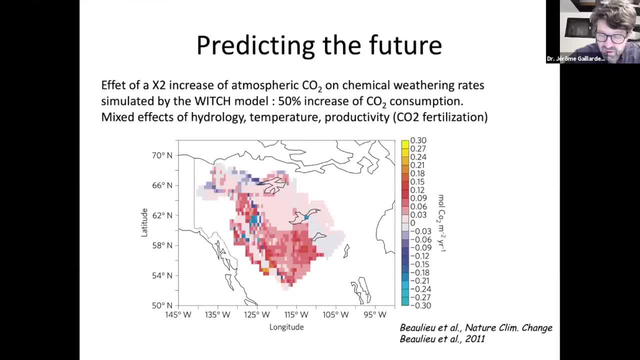 And, in particular, the type of study that I've showed you tonight is important. We need to know, to have a better knowledge of the different processes which are consuming or emitting CO2 on terrestrial surfaces, And because we need to be able to predict. 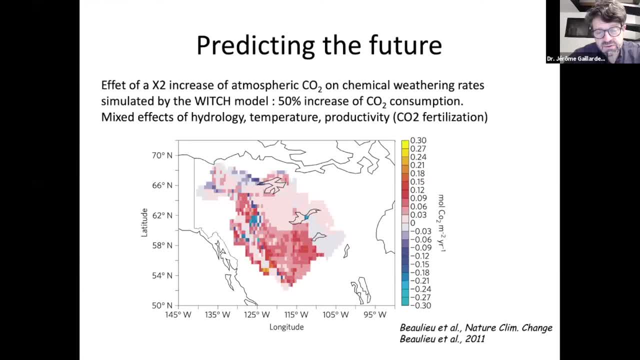 what is going to happen when the CO2 in the atmosphere will double and when the temperature will increase And catchments or watersheds like the Mackenzie River Basin, as you know, are going to warm up a lot in the future century. 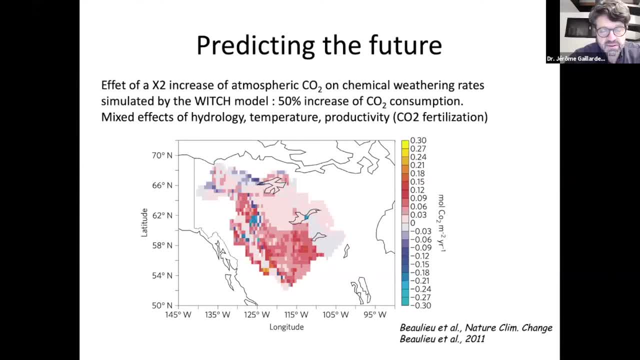 So this is really crucial: to better know what is happening today in order to be able to to predict. So this is really crucial: to better know what is happening today in order to be able to to predict. So this is really crucial: to better know what is happening today in order to be able to to predict.